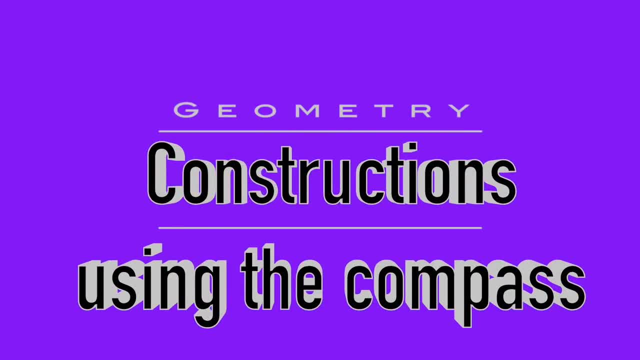 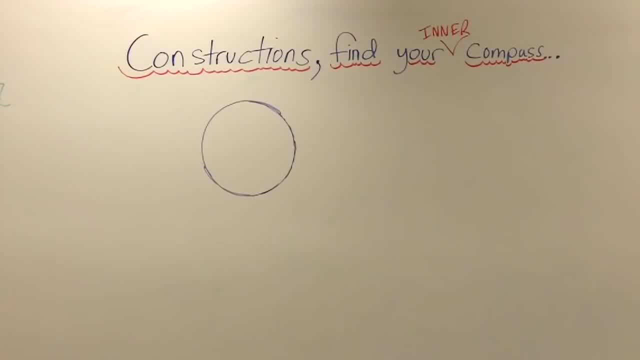 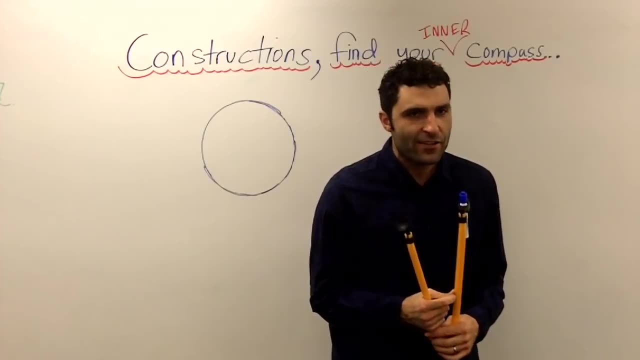 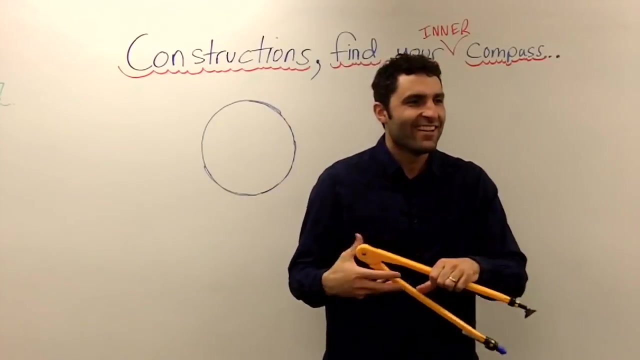 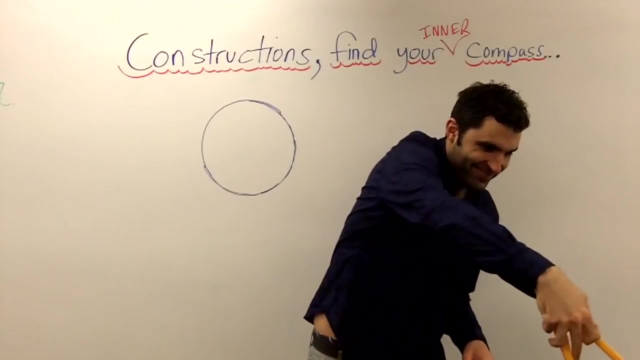 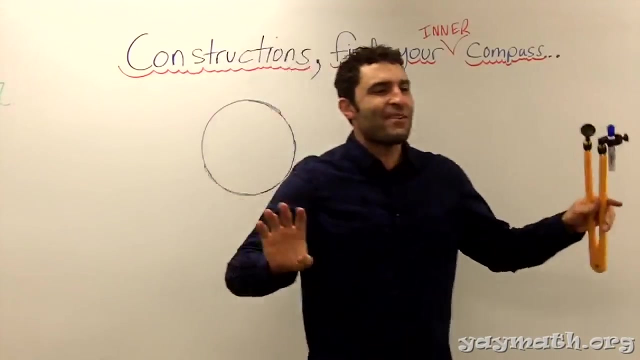 All right, everyone. Today we will be doing constructions with lines and angles. How do you feel? This is sort of like large chopsticks. I'll have the large roll. Yeah, we're filming. Yeah, that was a great moment. Now replicate it again. Okay, here's what we're going to use this. 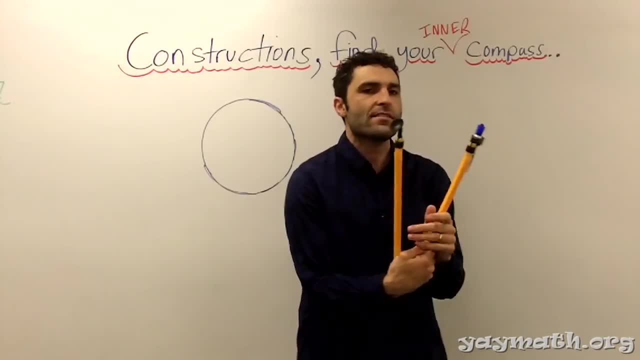 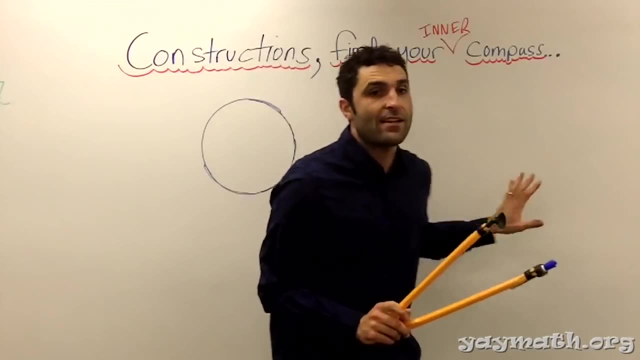 for? okay, The reason we use the compass is that it's a measuring tool. Yes, draw a circle. but not only does it draw circles, but it also allows us to recreate shapes like lines and angles and cut them in half. I'll show you what I mean. So you see, on your paper it says A, B, there. 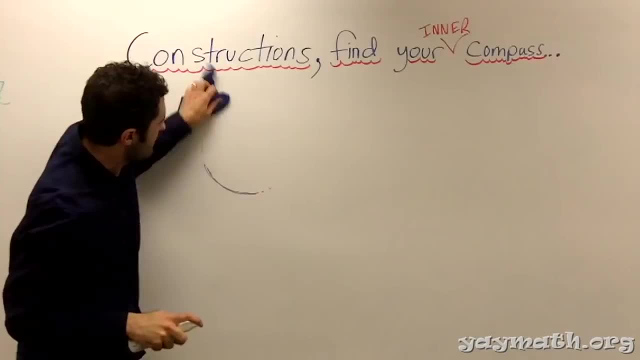 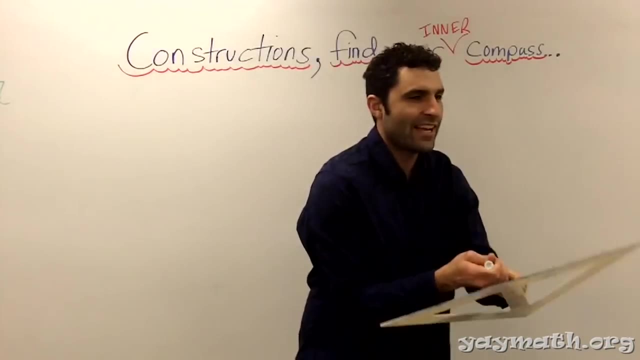 right. What we're going to do is we're going to recreate A, B, We're going to draw it again. I'll show you what I mean. So here you have. look at that. This actually flattens the fish. How does? 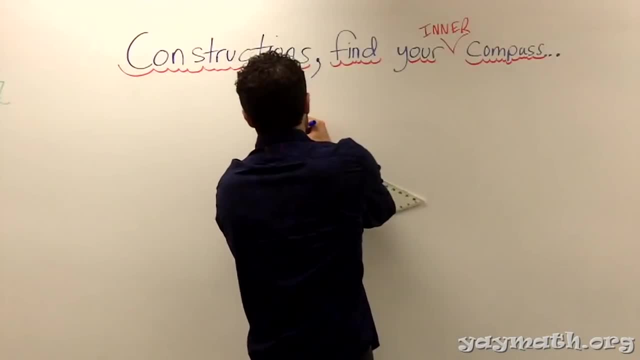 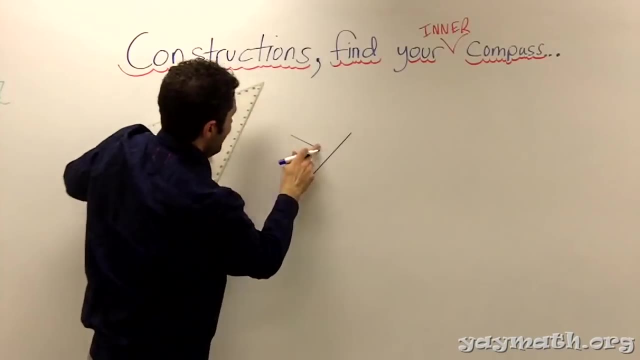 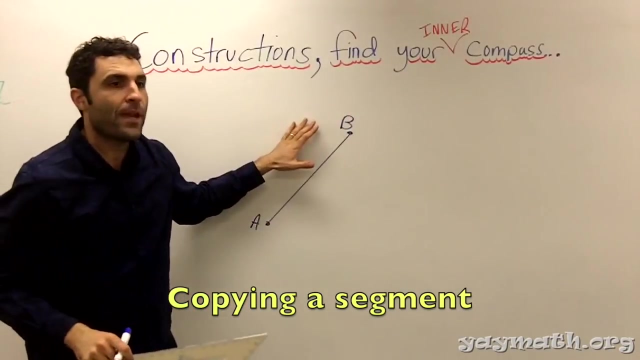 it. look on your paper, What shape Up there. like this Other way: Nice, Uh-oh, Uh-oh, You have to do it at a higher pitch. Uh-oh, Isn't that like a nap? Oh, So this is segment A B on your paper. We're going to draw another segment, exactly as. 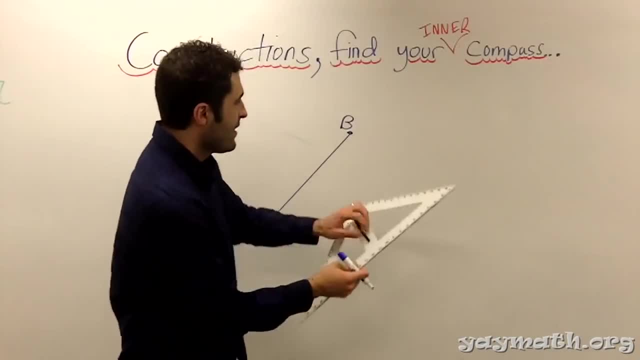 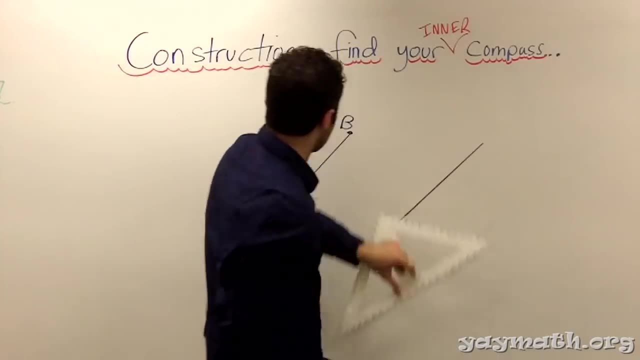 long as A B, without using the ruler, but using the compass. So what you need to do is take your protractor and draw a line like pretty long, longer than A B, Draw longer than A B. You can do that Like parallel. Yeah, you can do parallel to make it look nice. It actually 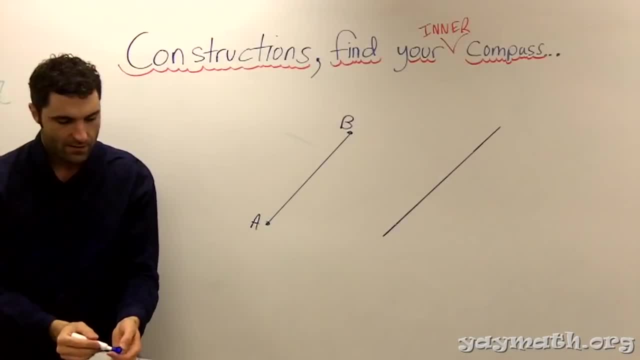 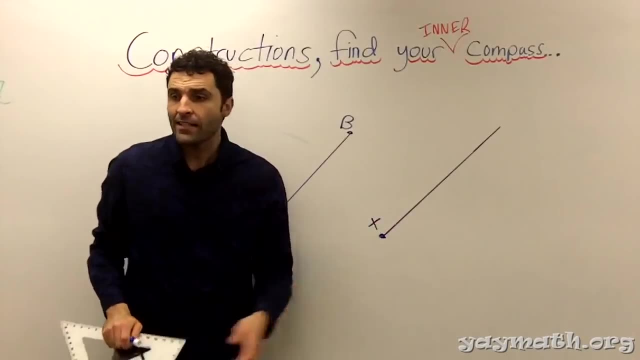 doesn't matter. It doesn't matter if it's parallel or not, And we're going to make it X, Y, Here, X, So Next to it, Yeah, next to it, Anywhere is fine. Now what we're going to do is use the. 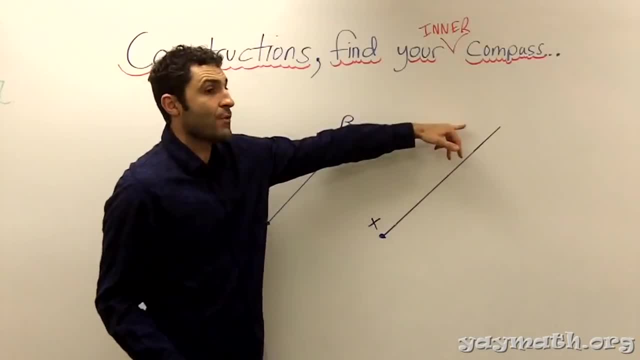 protractor. to make it straight: Oh, this is a protractor. Yeah, but we're not going to do Y. Y is going to be the end. Y is going to be the end. All right, check it out, We're going to use this. 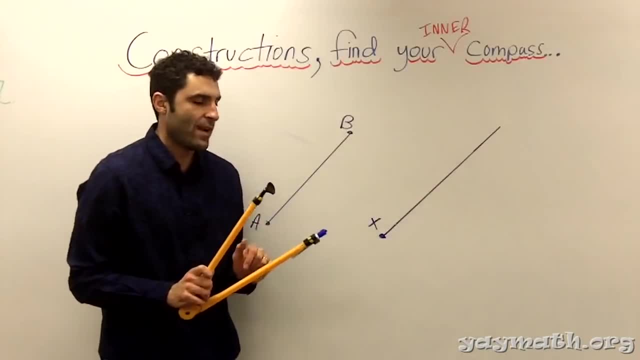 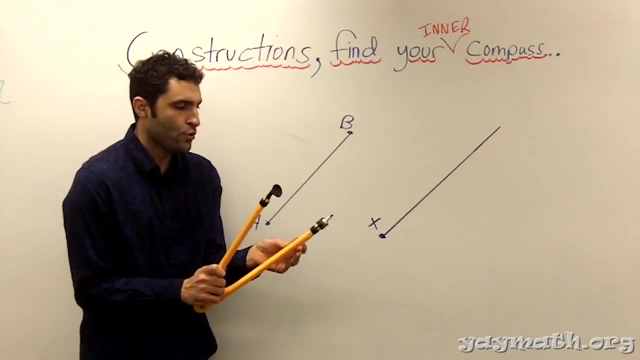 measure A, B and then recreate it to make X- Y. It's really not so bad once you understand the logic. So I'm getting a marker Ready, Okay. Rule number one: You can only make an arc at points. 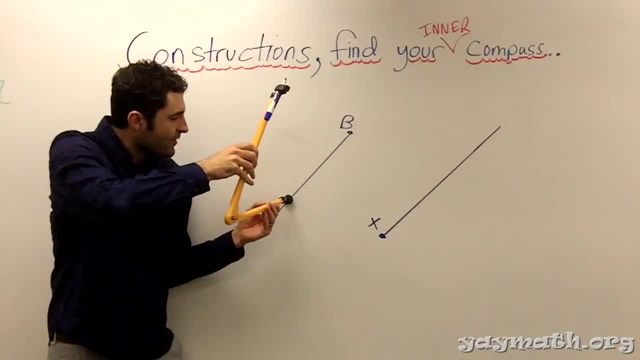 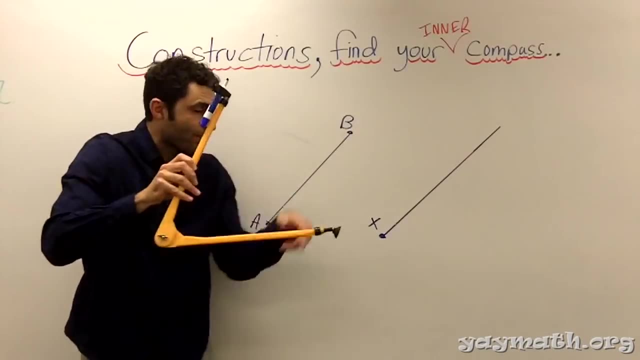 that exist. So I'm not going to ask you to make an arc, putting your needle anywhere in the middle of A, B, because we don't know what that is. If you put yours right here- and you put yours right here, you wouldn't know where they are. 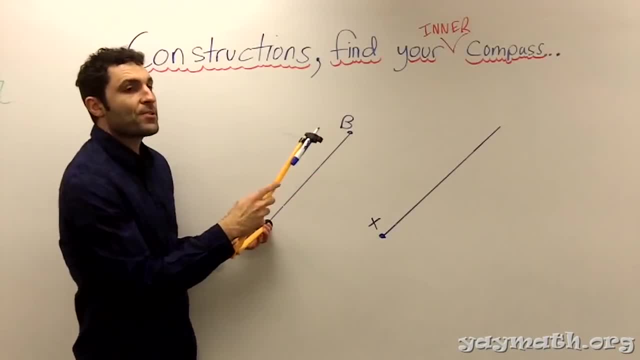 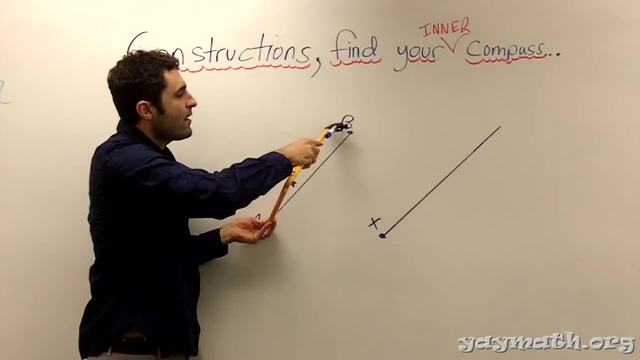 But could we all put them at A? So please put your needle at A, All right, And make a very simple arc right going through point B- Simple arc. You don't have to make the whole circle There. I made an arc at B. Try that. Yeah, I don't get it. Can you put your needle at A? 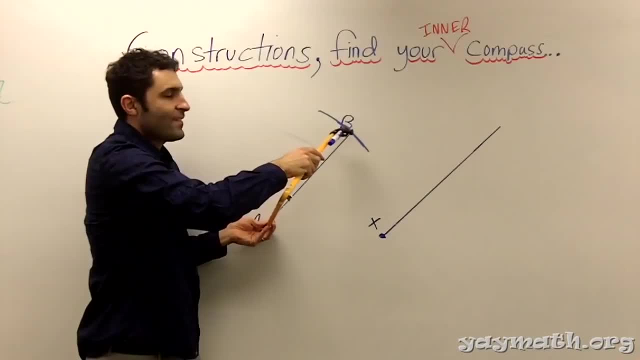 My needle at A. Yes, Very good. Can you make an arc? How far down can I go? It doesn't matter, Not far at all. Through the other one. No, Oh, No, You're just measuring how far A to B is. 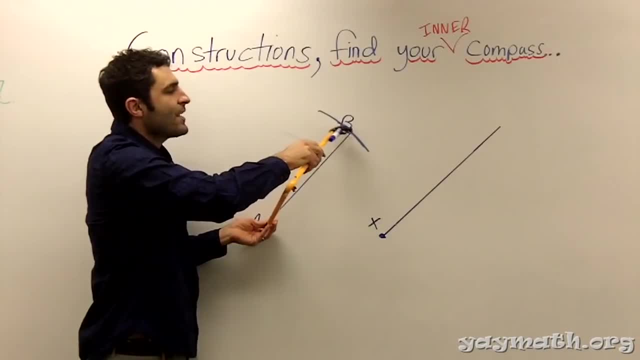 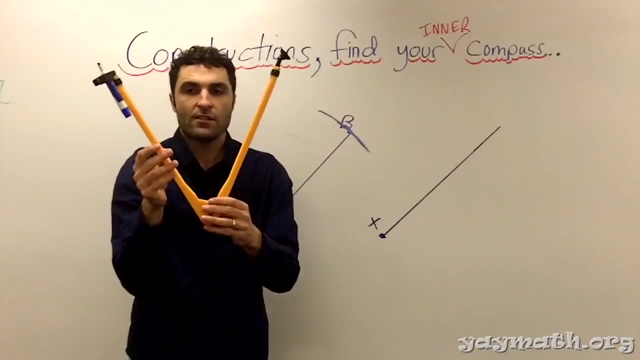 Oh, Does it have to be exact? As close as you can through B, And then, once you have an arc through B, you keep the compass where it is. It's rule number two: Don't change the length of this radius here. 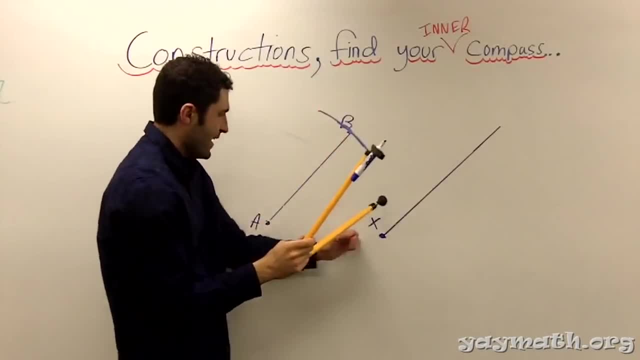 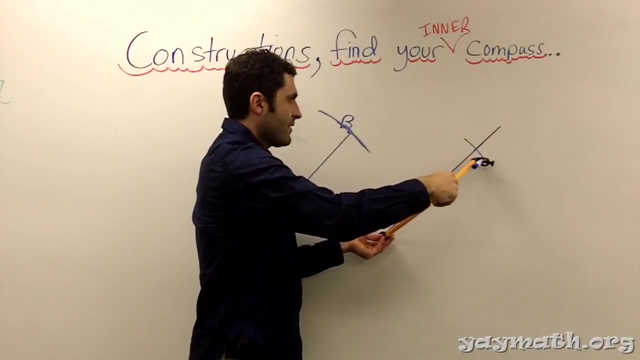 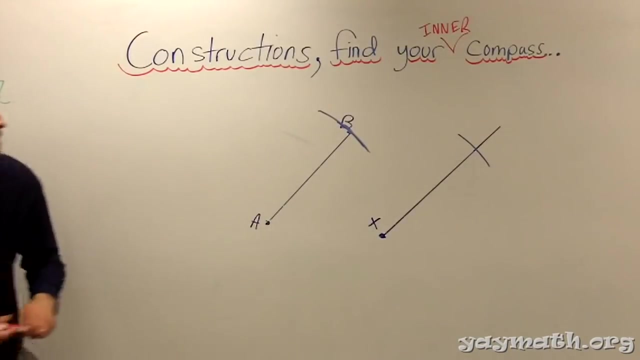 And then put the needle at X, sort of like what A is. Put the needle at X and create the same length arc. Oh, I get it. And now we've just recreated AB. Wow, They don't look the same anymore. They should You have to imagine it. 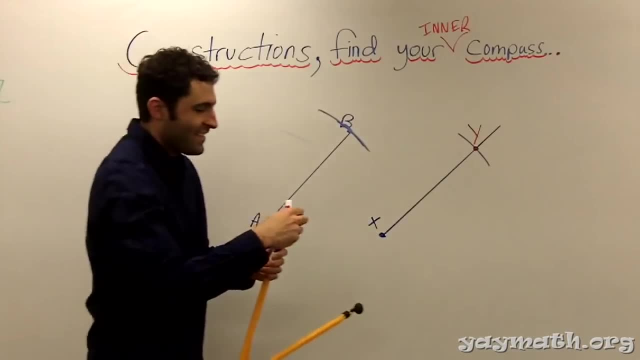 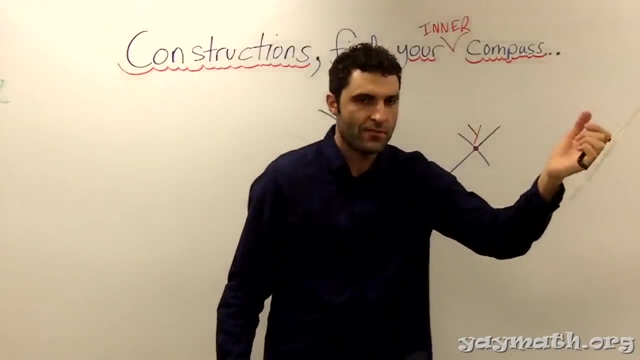 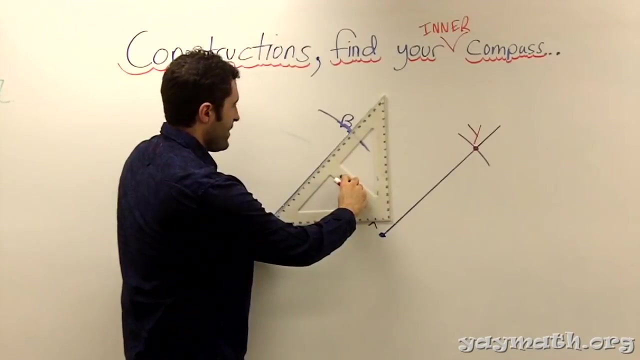 Hopefully our imaginations aren't too active and that they're actually the same. Now let's verify, using your protractor as a measuring tool. So for me, I have. I'm at like 17 inches. For me, I'm at 17 inches. I'm going to go over here And it's the same. It's the same 17 inches. 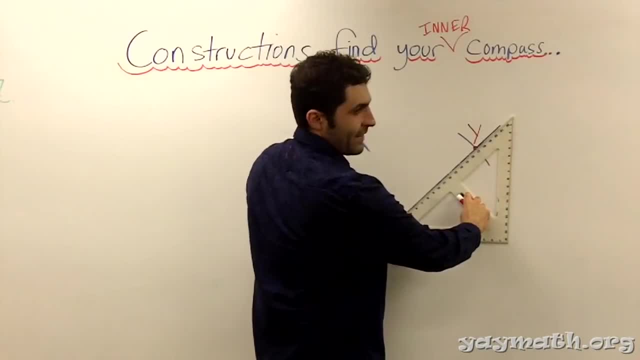 Whoa, How about six lines? It's the same. That's so cool. It is pretty cool. We're only getting started. That's so cool. We're only getting started. Okay, flip the page. Wait, wait, wait. 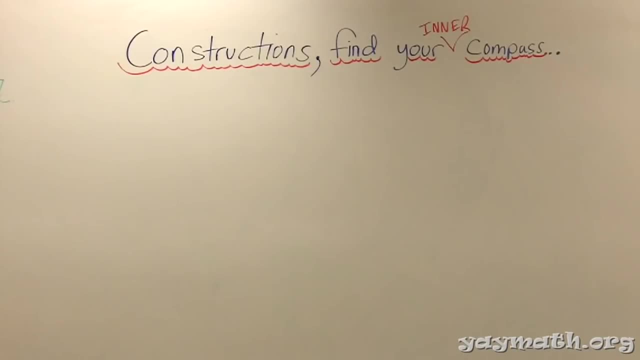 All right, You guys are on the same sheet. I'm having fun in them. The little side, The inside. That's why it's called yay math. Say it with authority. What? Ah, Those are seven. I'm having fun in them. 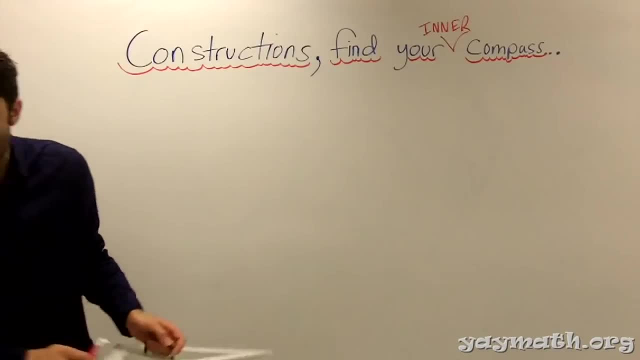 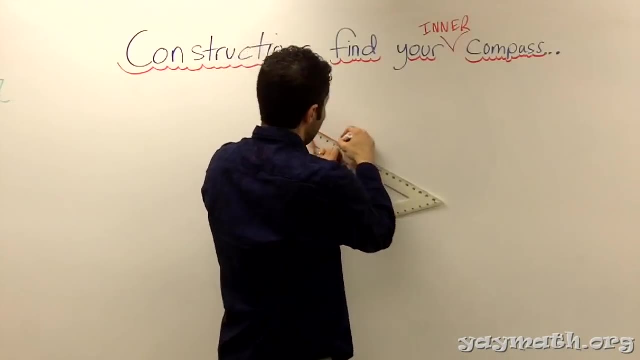 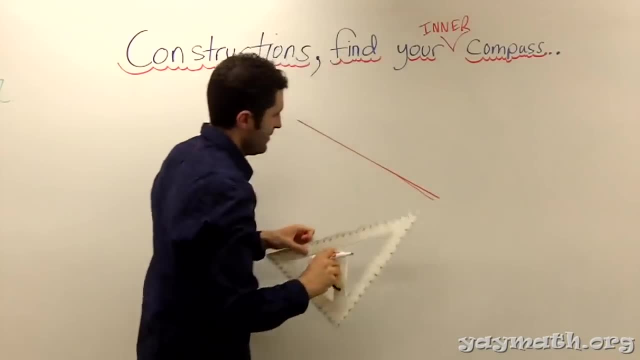 The two Said with authority: Ah, Those are centimeters, They're smaller. Yeah, it's one. Guys, don't complain to our camera. God, All right, good job. Here is PQ. Can we do the same thing? 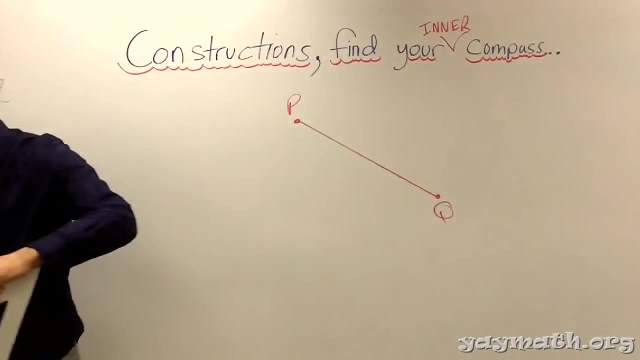 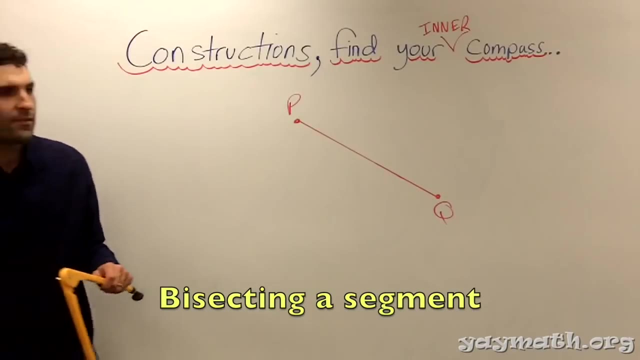 No, now we're not recreating the line. What does it say at the top of this page? Bisect— Bisecting a segment, Bisect. What does that mean? Anyone? Cut it in half. Cut it in half. 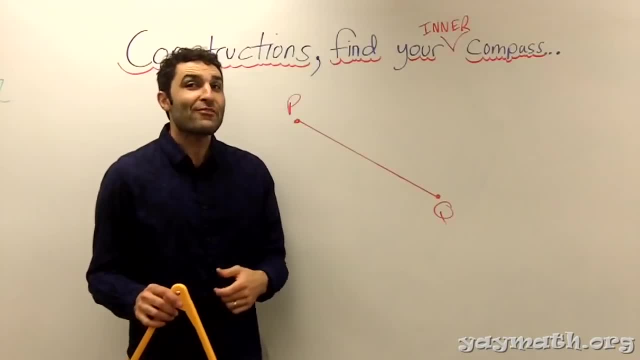 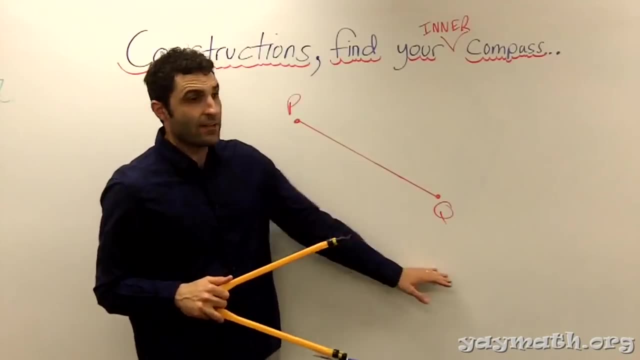 Cut it. So now, Pop culture references. if we're cutting this line in half, do we need to actually make another line? or just cut this in half? right, we're just cutting this in half, okay. so back to rule number one. what was rule? 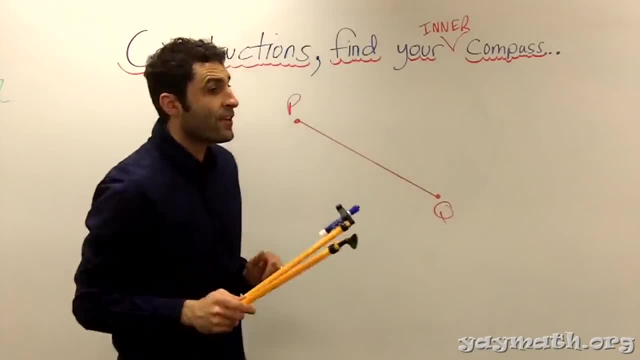 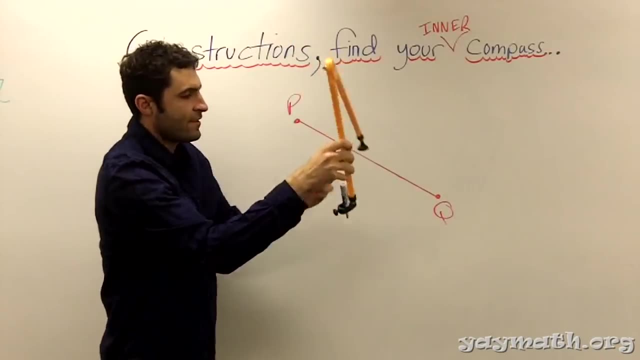 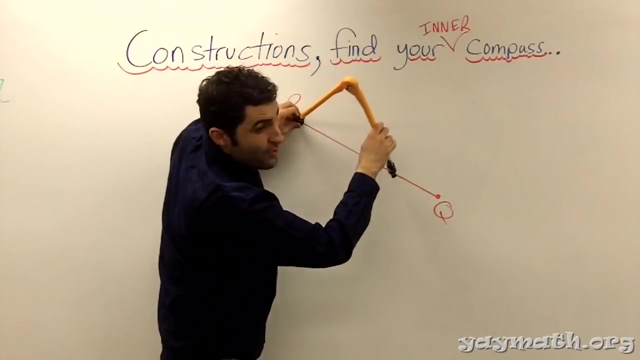 number one: where can we put the needle on a point that already exists? let's go ahead and put it at P, okay, and what you want to do is: you're gonna go more than halfway from the line. more than halfway. no, not always you, although you could actually- but it's not necessary- go more than halfway, and 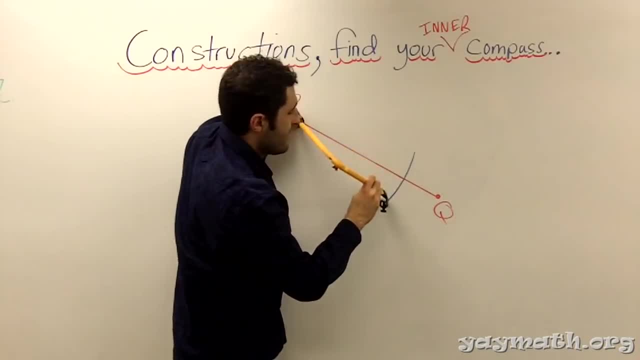 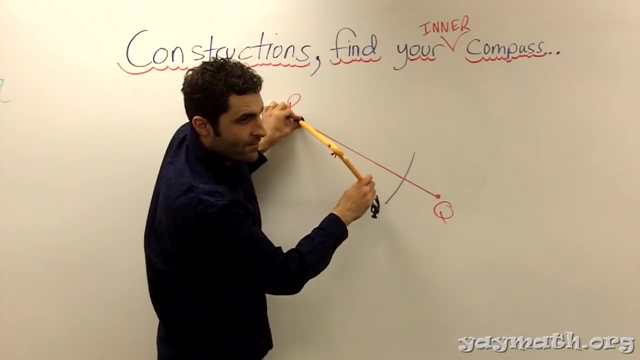 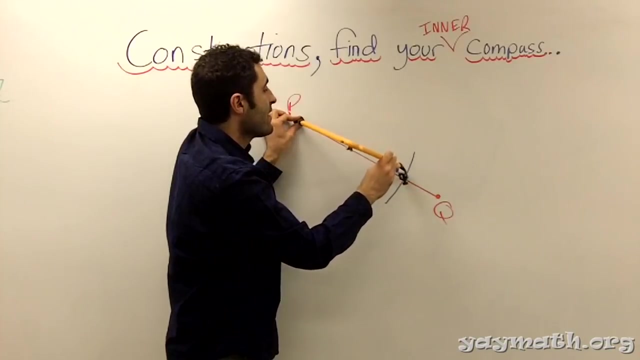 I gave us a little arc. okay, starting at P, more than halfway to Q, and aren't there? no, no, it's not too precise, but once you pick your measurement, you have to keep your compass the same. that is rule number two. number two: now that I've made my arc, I'm not going to change. 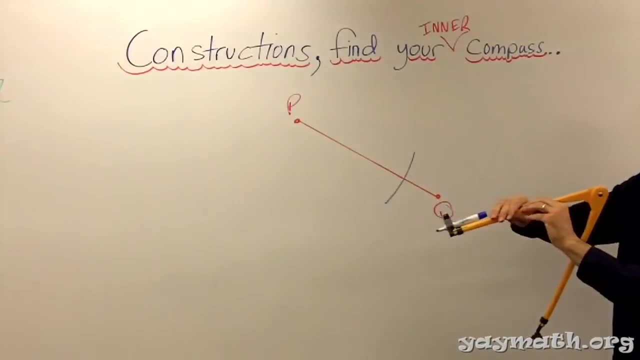 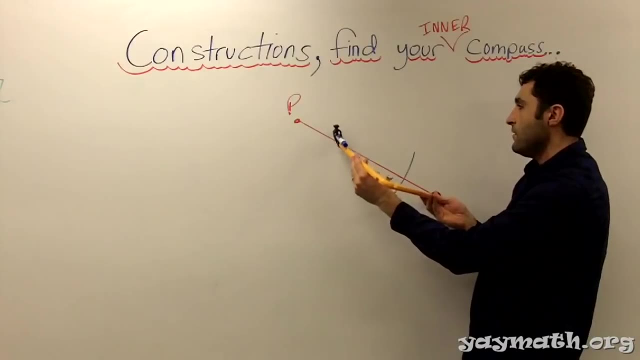 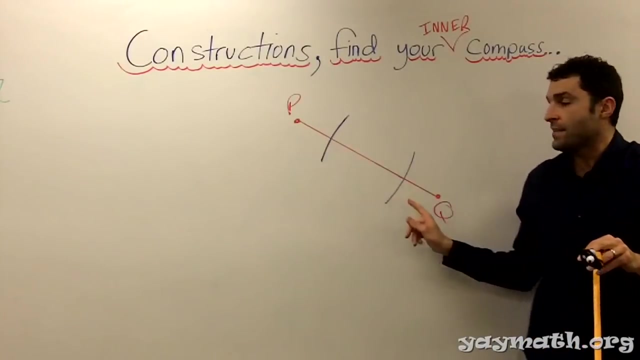 I'm going to bring my little violin type of thing and do the same thing. from the other side it feels like I'm doing violin. wait, how do you find the half? we haven't done half yet. so what is this? remember the arc that we created from key to half, all more than halfway to Q. 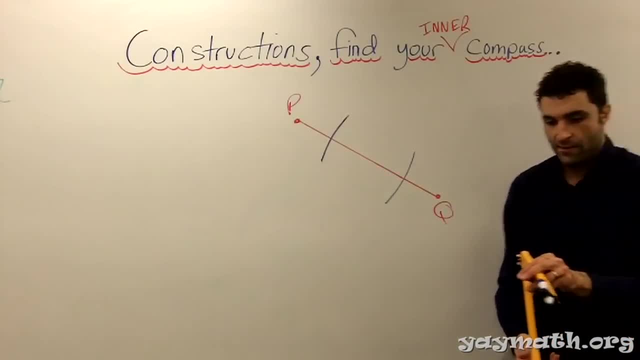 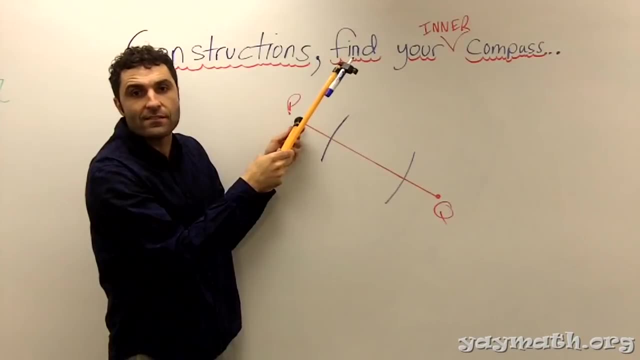 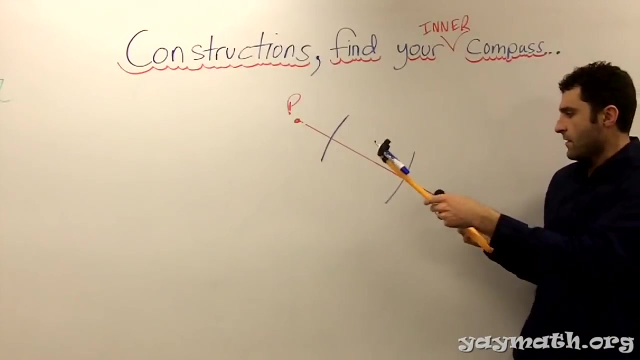 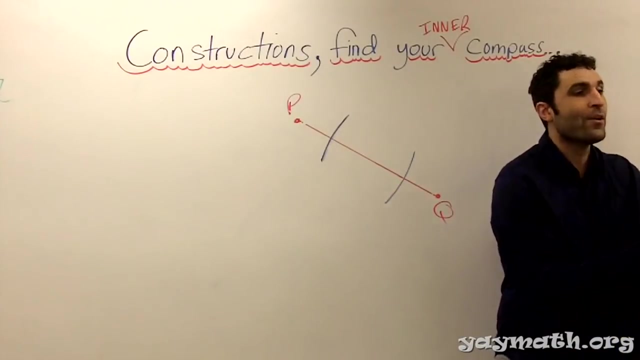 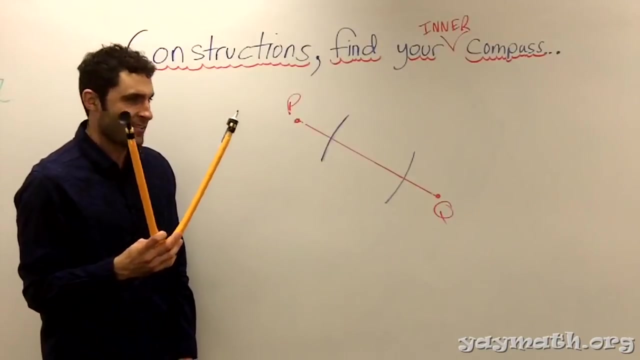 this way, do you have to choose a a certain length? nope, nope, everyone can have different lengths. thank you for asking. so we did this art the same as this art. okay, now back to rule number one. rule number one is: you can only put. I count how many new points created. two, boom, that was awesome. 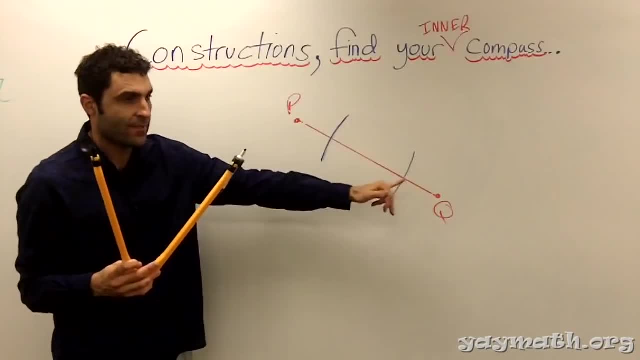 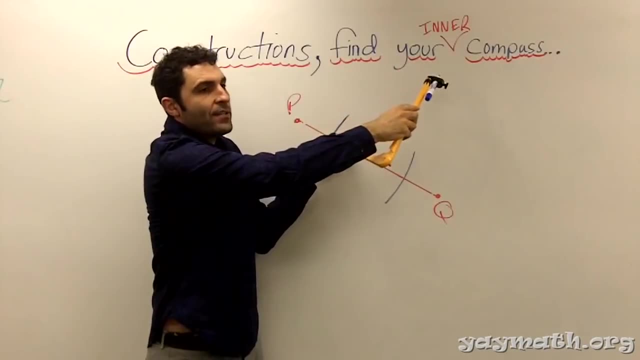 wow. so now we can put our needle there and we'll put it here and there. so let's go ahead and put our needle there now, without changing it. now, look, you're welcome to leave it what it is or you can change it. now we can change it. we're starting a new round. if you leave, it goes all the way to Q. 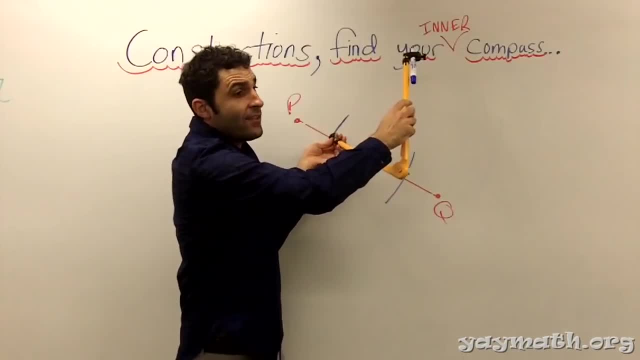 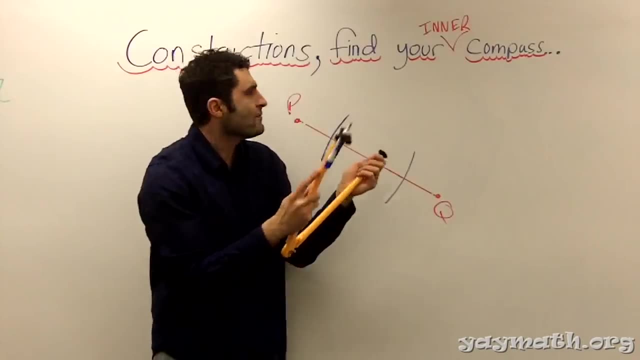 I think that's. uh, yeah, it does go all the way to Q. yeah, that's true, you can leave it. we're not going. we're not going to Q. we already know that it goes to Q because we started from Q to there. so I want to change it, so you can. yeah, I would like you can make it a little longer. I don't get it all. I'm asking. 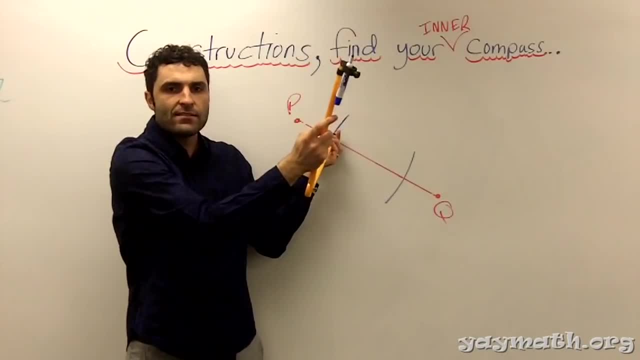 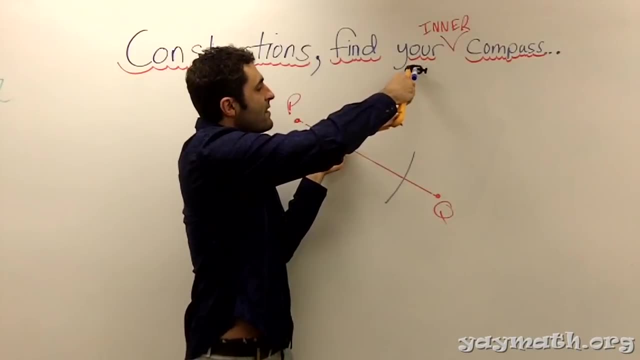 you to put it on this new point, and you can change it. now it's okay, make it shorter or longer, uh, make it a little longer. and then what do you do? I'm about to tell you now, come out in space. so right, where the midpoint, the middle line would be, give us an arc out here in space. 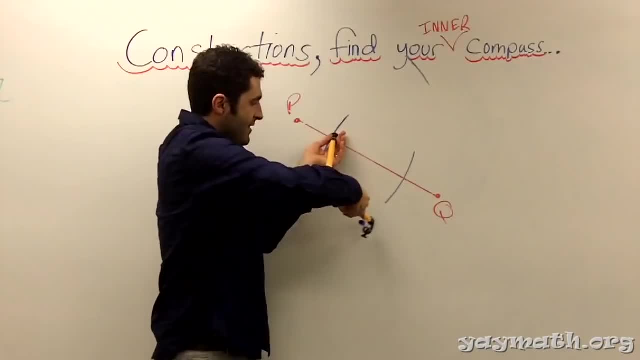 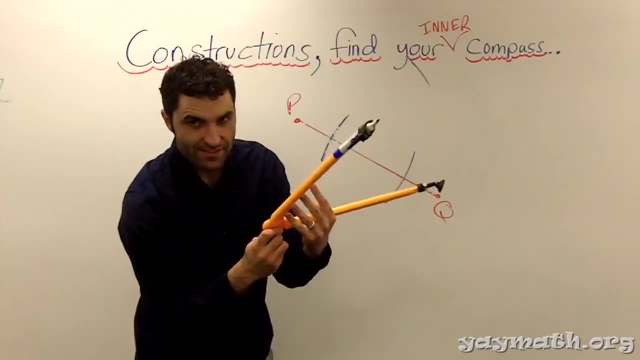 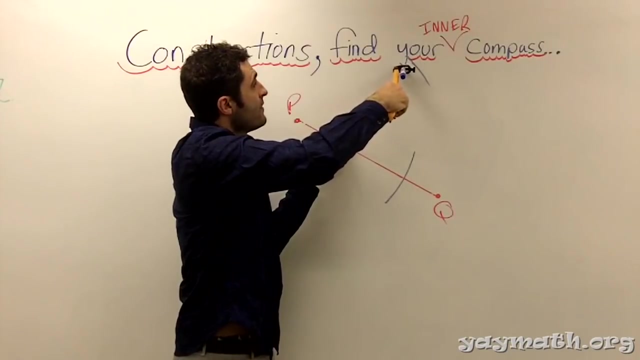 okay, and then and then do the same thing below, except I didn't lock them. I need to lock it up. lock it up. how do you lock it? I'm fine, no, no, don't make a circle all the way around. although you could, you could do that, so I messed. 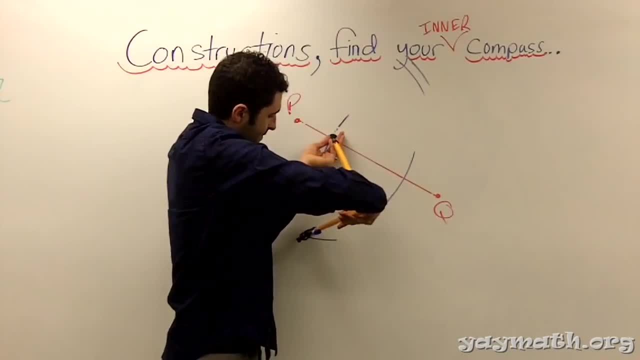 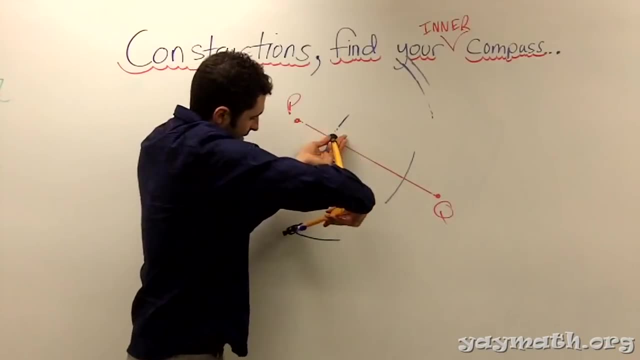 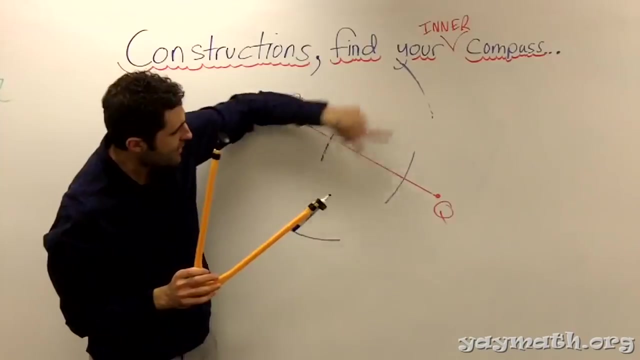 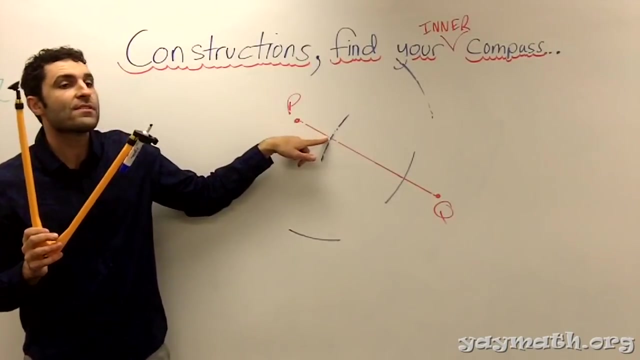 mine up, so I'll do it again. I'll race there. so you're going up and down. two arms here, one and another here. so this one was wrong. okay, so I have one arc up here, one arc down there from the new point. now we'll get it. now we're going to do the same process with the same length from the other point. 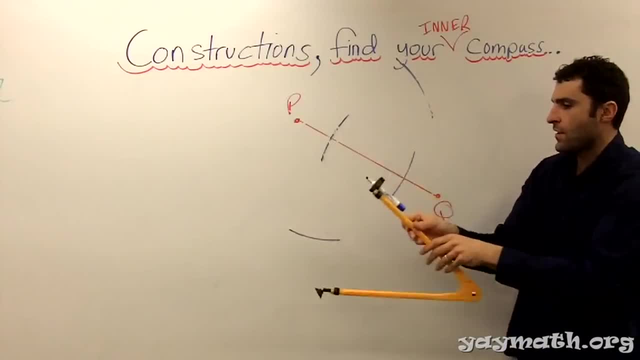 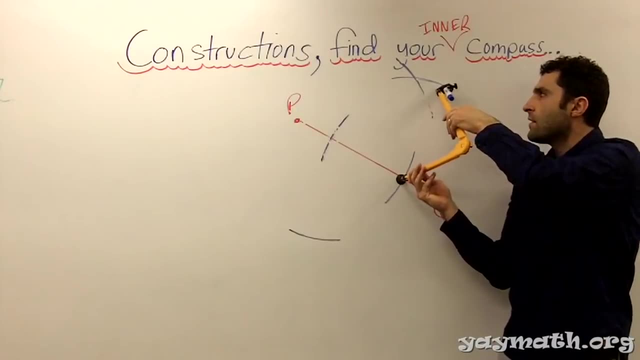 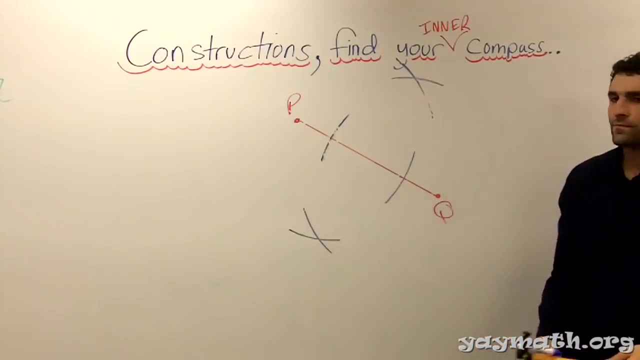 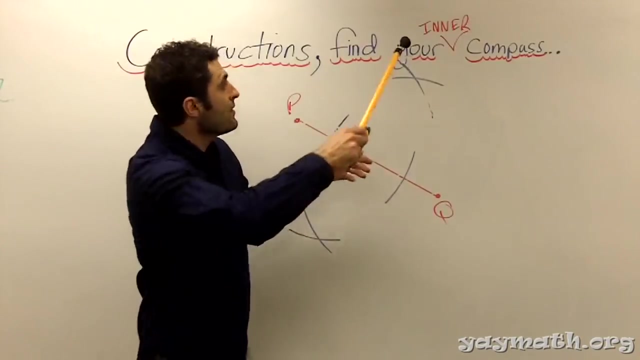 so to bear with it, and you'll get it there. it is, oh, over here. new point: same concept here and now. mine doesn't touch it, okay, oh, it wasn't long enough for them to touch. oh, so you may need to say so. either either you need to increase the length of your arc or you need to continue drawing. 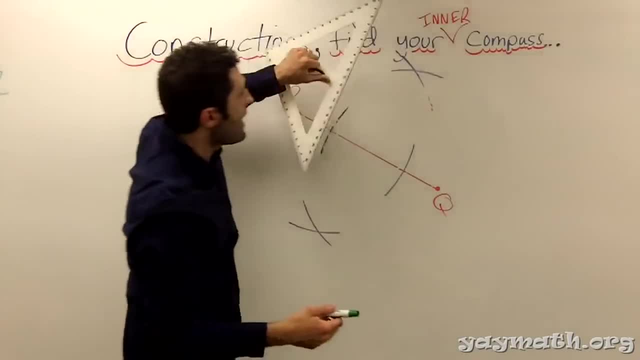 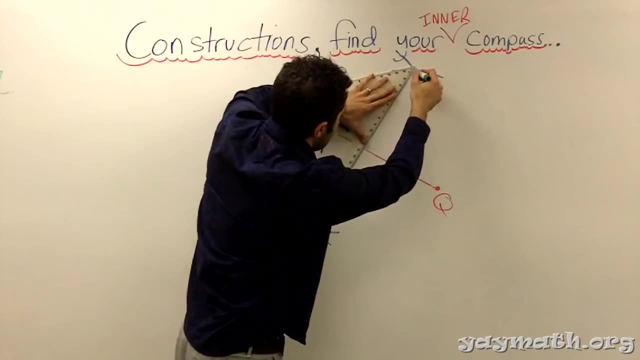 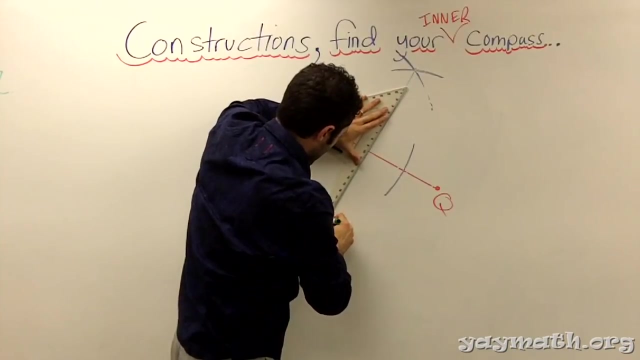 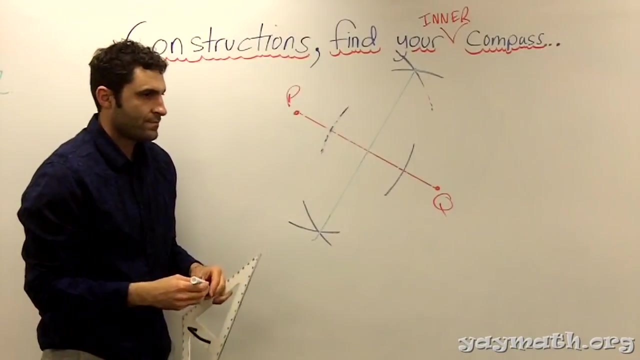 it until they do okay, oh, and then observe: connect the dots, connect the dots. what can you do? just gone from Q up and then from P, I'm gonna ask you where the dots ask the question again, sorry, And then I just have to put my thing on cue and draw it up and then my thing can be screwed up and connected to the door. 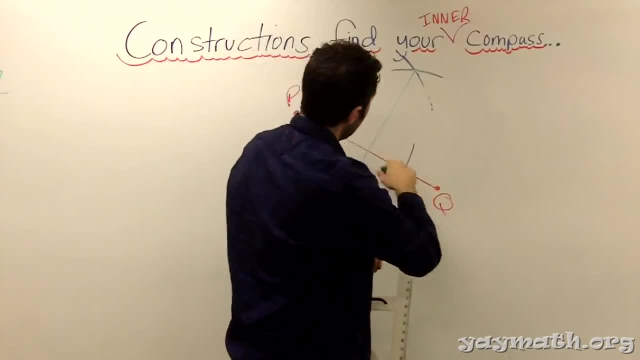 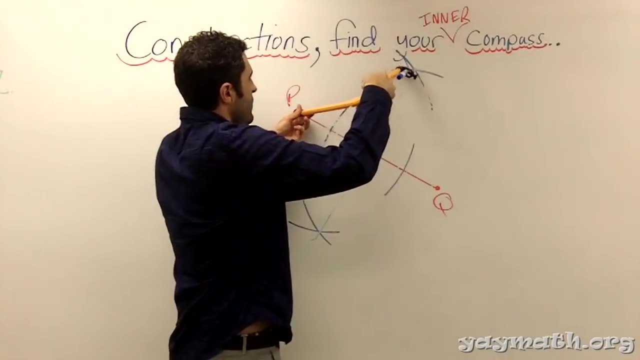 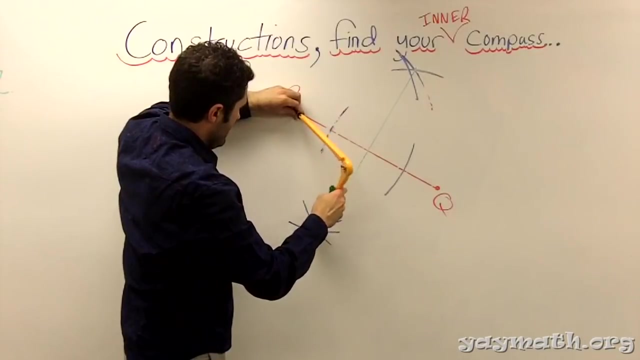 Half of the length of the thing in cue. Whoa, I give up. Okay, so that's what you said. You're contending we go like this: One, Two. Can we switch papers? Why? Because I'm on cue. 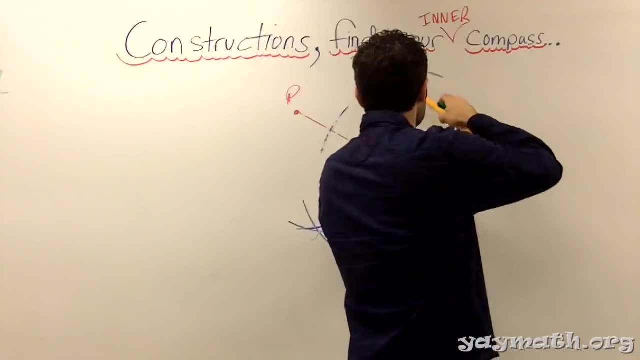 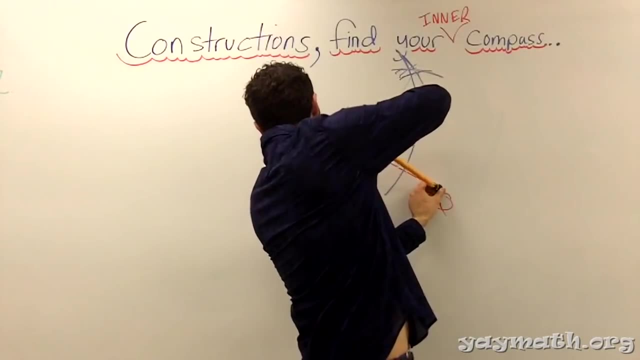 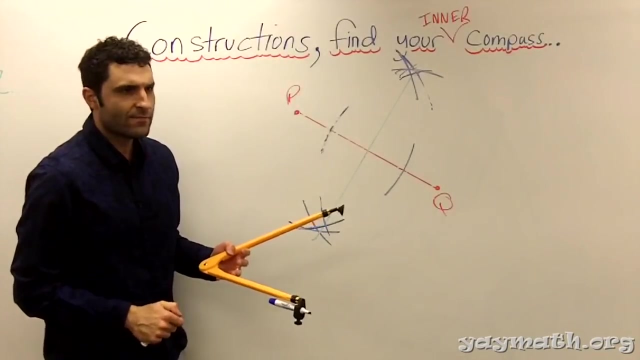 One, two like this. I did it. Yeah, I think that would work too. Is that so much simpler? Yeah, Yeah, I created an additional point needlessly. You want to do it an easier way? Let's do it an easier way. 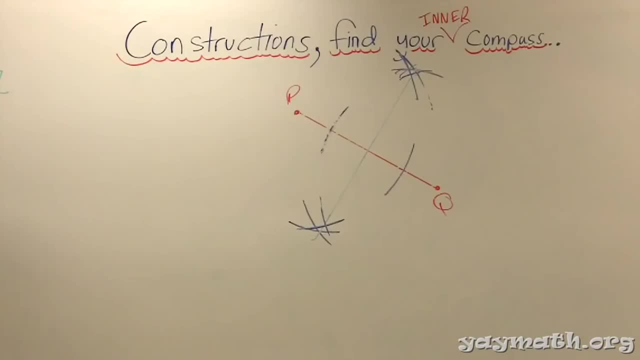 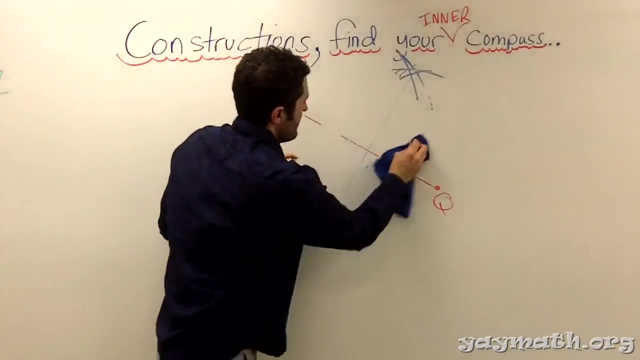 Wait till you got make one. Should I erase this? Yeah, you can erase. I kind of like it. I think it's pretty. I want to do the new way. I'm going to delete, I'm just going to draw a new one. 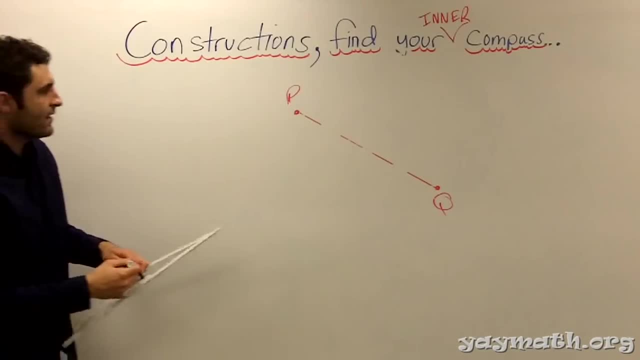 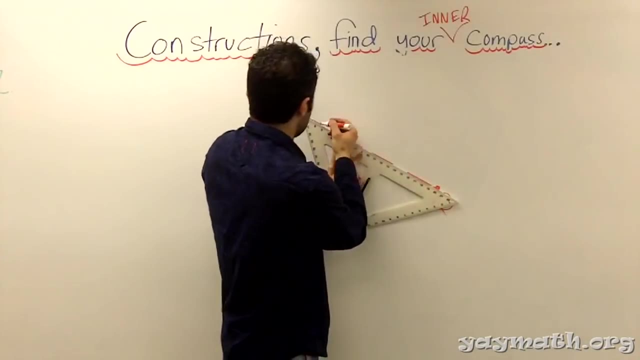 That's a good idea too. So you have two methods for you. I'm going to draw a smaller one, Smaller ones also, So you have like two different concepts. We're going to do the Carmel method. You can't say that on camera. 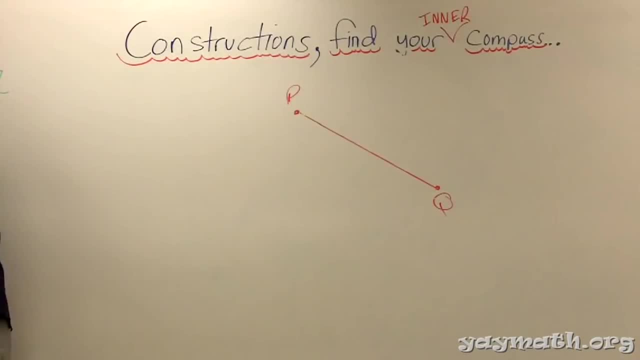 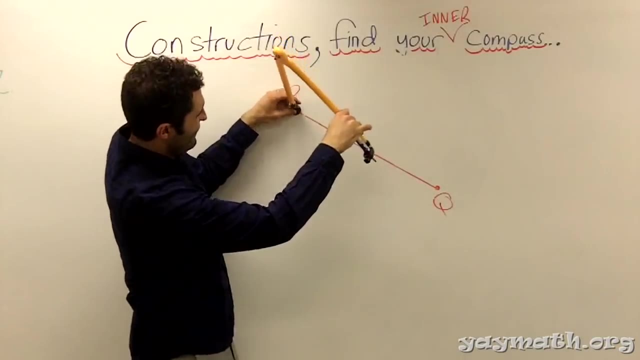 Oh, we're going to do the Carmel ice cream, The Carmel ice cream method. Yay, Carmel ice cream. This isn't going too well. This is going awesome. So we pick a point and we go out in space. 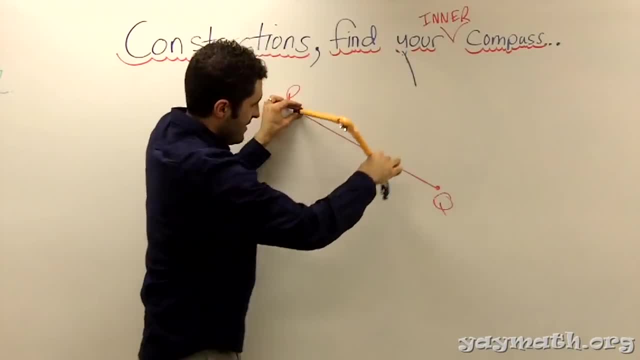 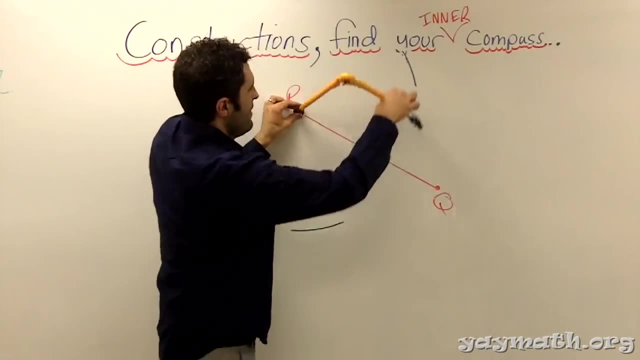 Out in space one. Space Out in space two. Out in space two. Oh wow, it's so much better than mine. Yeah, Wait, what? Out in space one? It doesn't matter how far apart it is, As long as it's more than halfway. 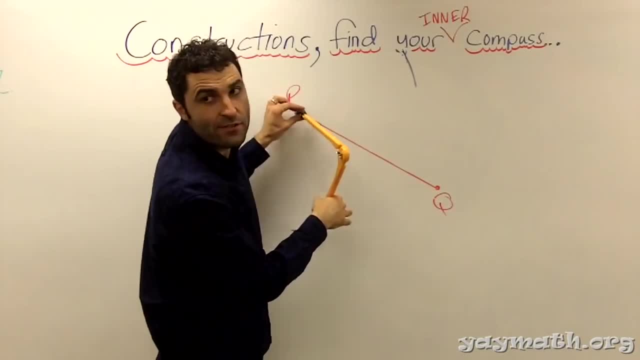 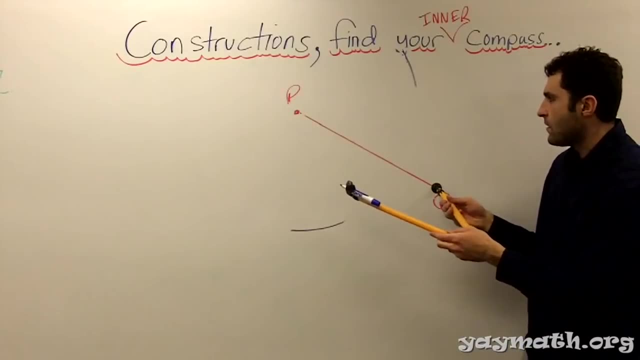 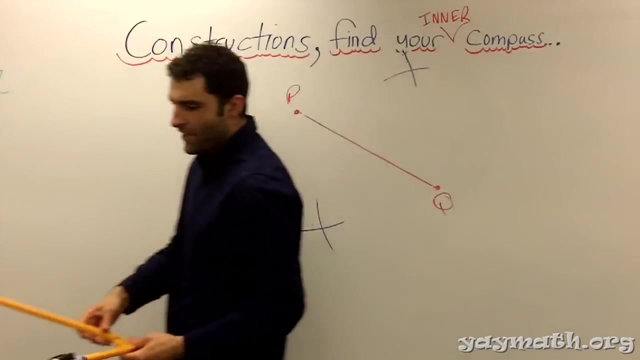 Okay, Out in space one, out in space two, and then recreate process type. I'm just going to keep my first: one Okay, Out in space. one out in space. two out in space, two out in space two. Oh, it's so good. 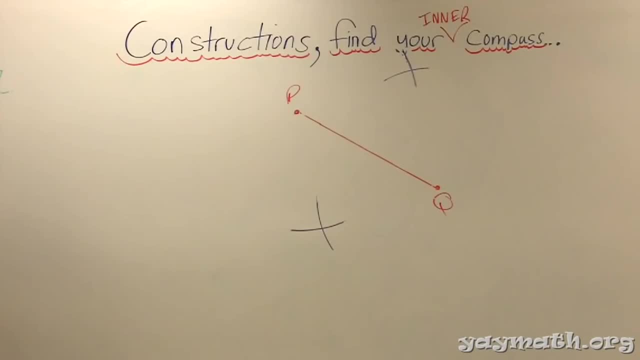 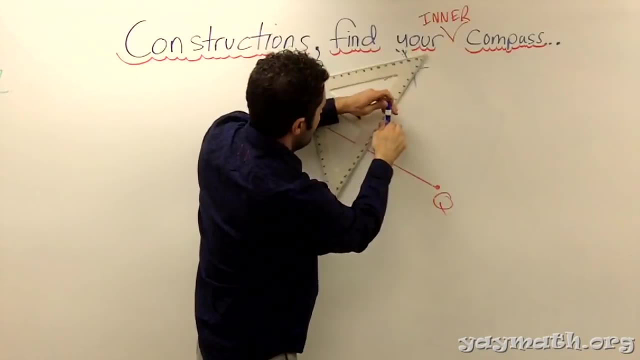 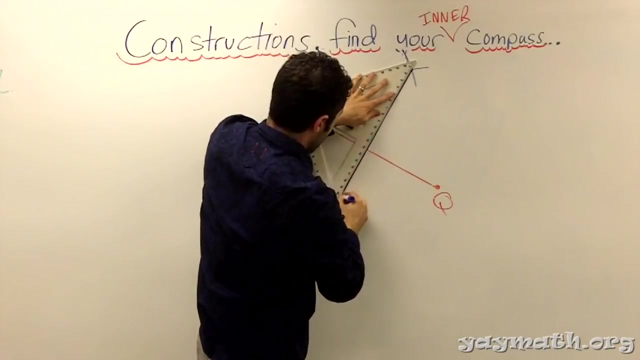 And now it is bisected. Wait, can you explain what you did? I just did, I didn't create a new one. There's two set of points. Was that your flesh? cutting under the point, though The compass Me No. 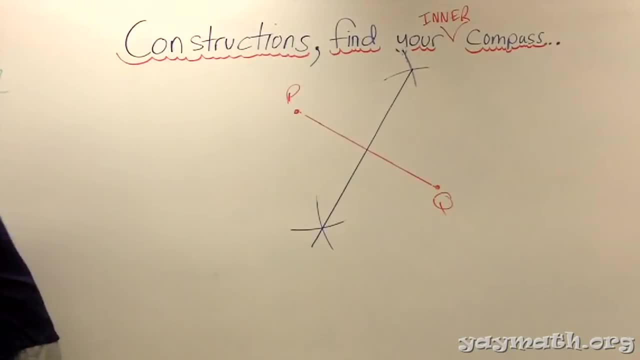 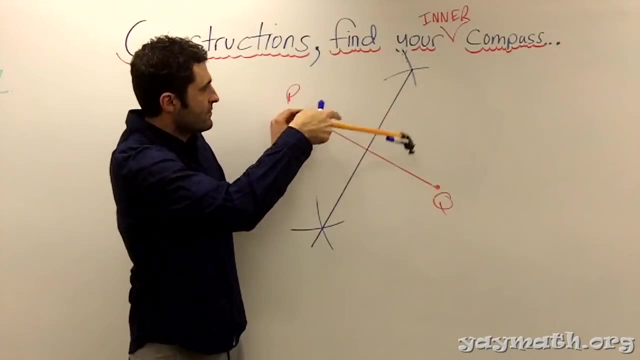 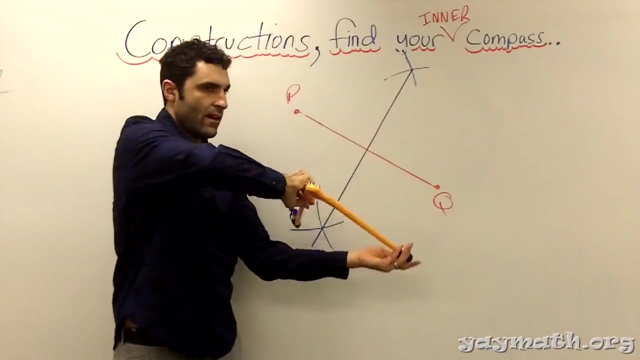 Okay, I heard like: ooh aah, What we did, sir. start here, create a point, create two arcs, arc, arc and then over there, arc, arc. Good job, Awesome, Yay, Matt. 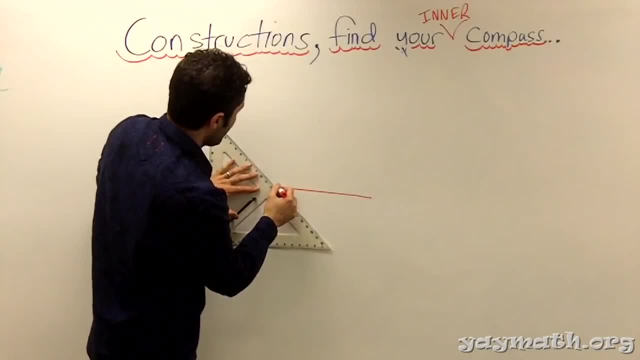 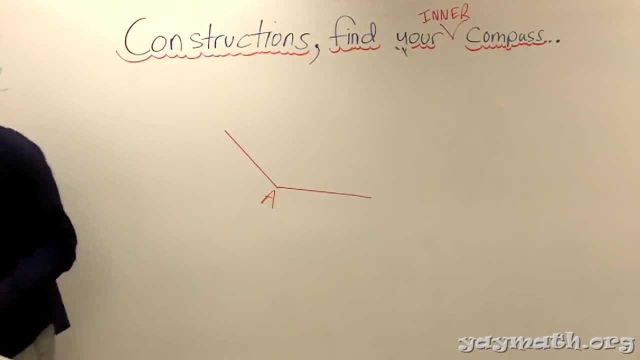 Don't you know the right beat? That's the wrong beat. Don't you know them? That is the right beat. That is the right beat. You should have cheerleaders. What are we going to do with this angle? What's it say? 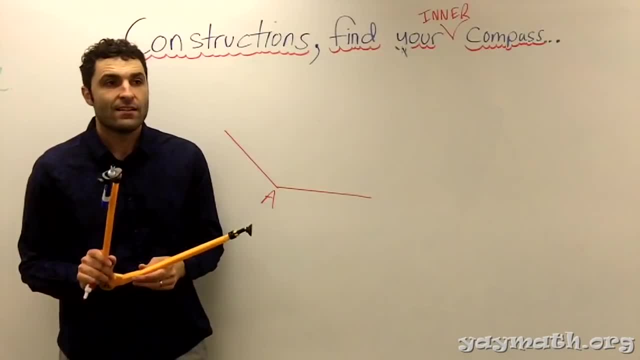 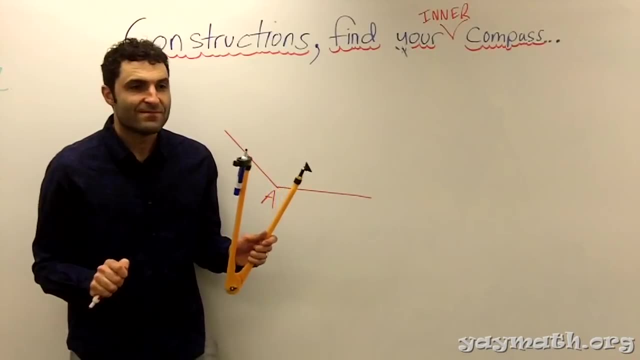 Cry Or disrupt. I'm still sloping for that A congruent angle to A Oh wait, This is not. we're not going to have a test or a final. Oh, my goodness, Because I do not need to do it. 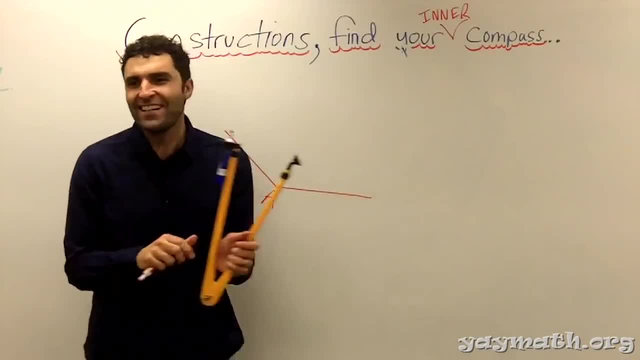 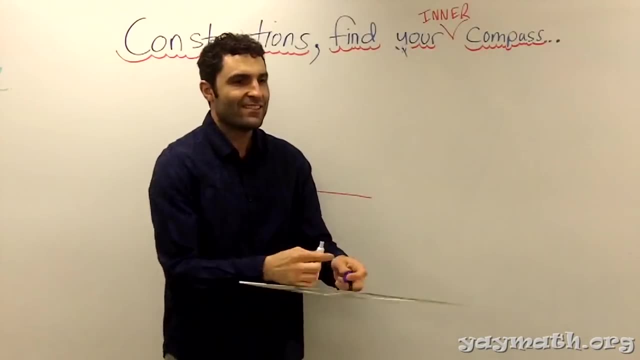 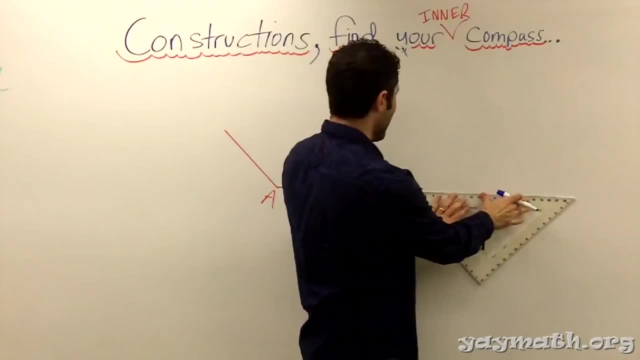 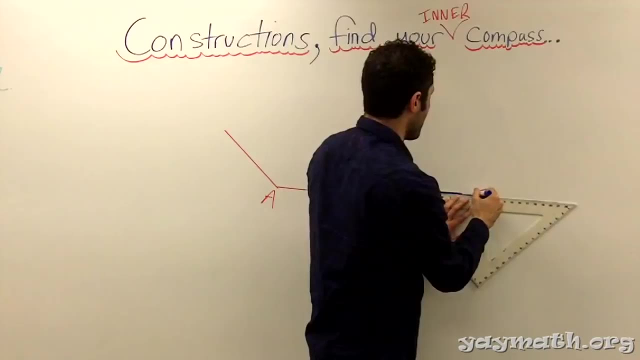 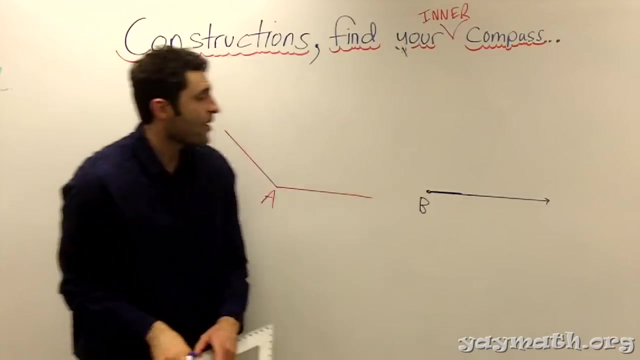 Let's call it angle B. We're having a good time, it's true? No, don't use the projector. Use the projector to verify What Wait? should we draw that? Yeah, So you're drawing. We're going to make angle B. Notice, it's not ready. 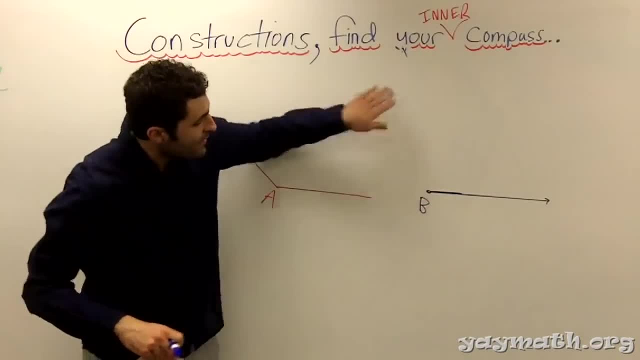 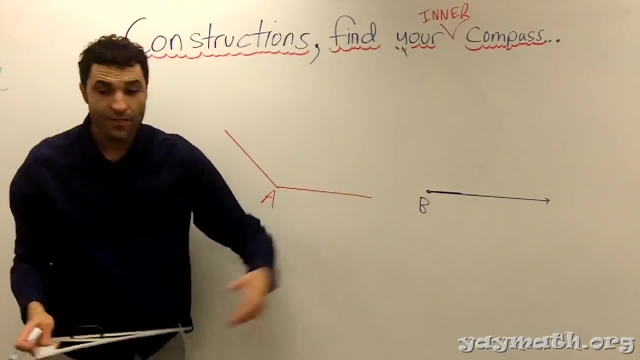 Alright, it's not ready. We don't know where to draw the new line yet. It's going to look something like that probably, But we don't know what the angle is until we use the projector to measure it. Why did you draw that line? 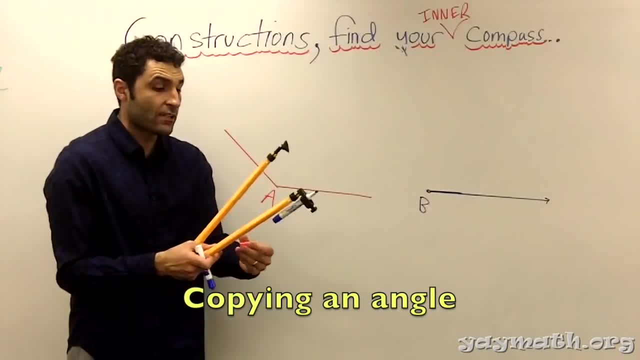 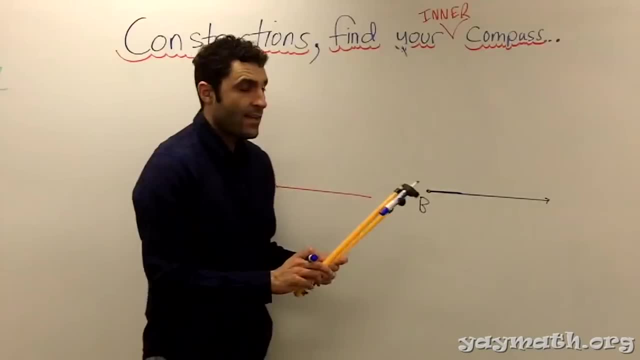 Because we're going to replicate it. We're going to make an identical. How do you draw a line? We're going to construct, We're going to construct. Does that have to be the same length? No, good question. It's not going to be the same length as long as the angle is the same. 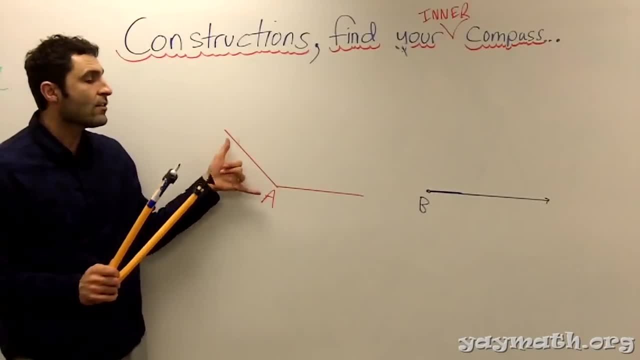 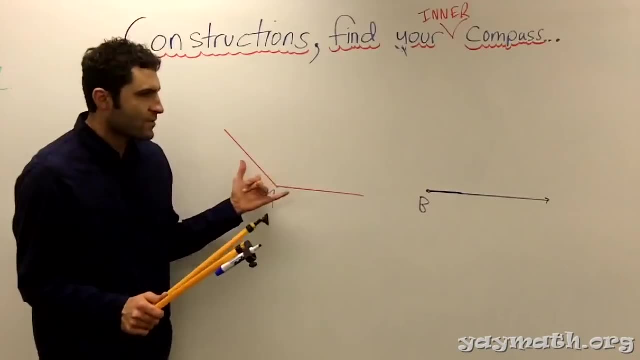 I can take this off a little if I want. It's not about how long the lines are, It's about the angle. Like, tell me about the angle, Is it acute, obtuse right, Obtuse, Obtuse right? So we want to know if our angle will be the same. 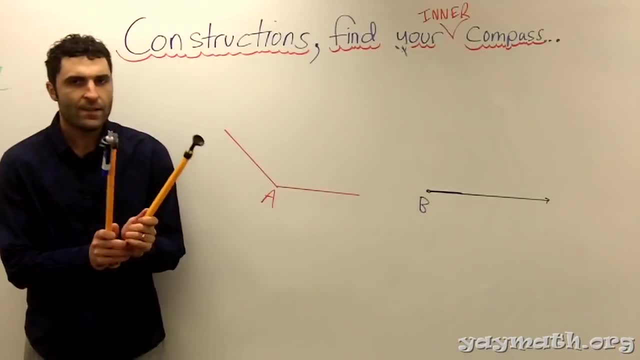 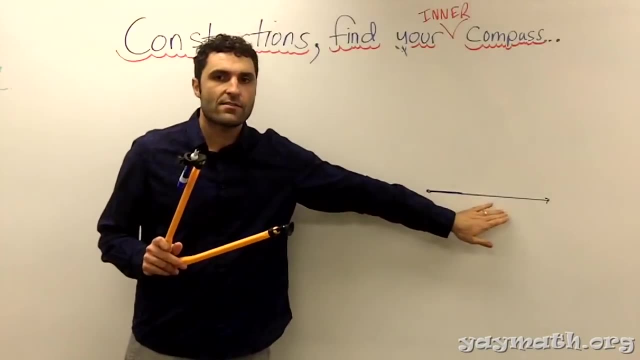 Not necessarily how long the lines Got you. Okay, Do we have to measure it? We will after with the protractor to verify. So are we supposed to draw the B, Draw the new line? yes, How come we can't just measure that one and just redraw the same? 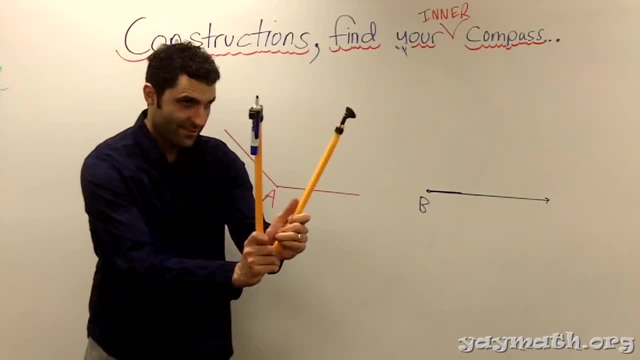 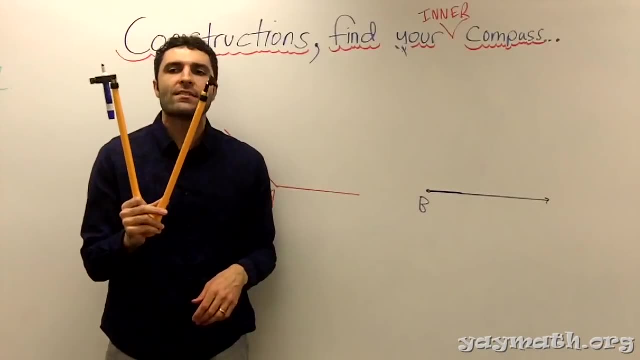 Measure with what? The protractor, Yes, The compass, Use it with this, Try with this And then confirm with the protractor. Okay, I'm with you All right. So rule number one: where can we put the point always? 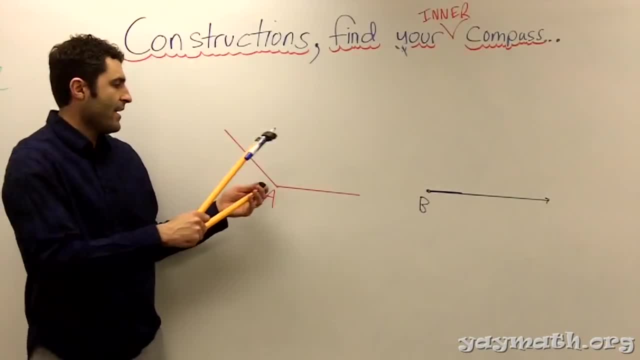 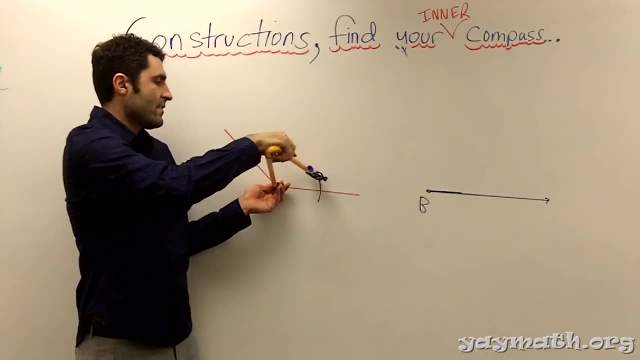 On another point. On another point: What's the only point that works? A, A, A. Give us an arc that covers both rays. Huh, That covers both lines. It has to go through. Yeah, No, It has to go. 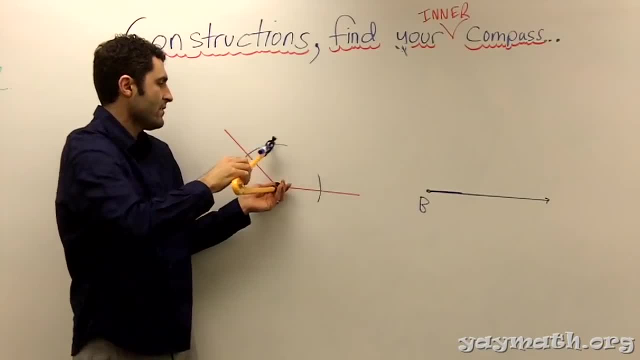 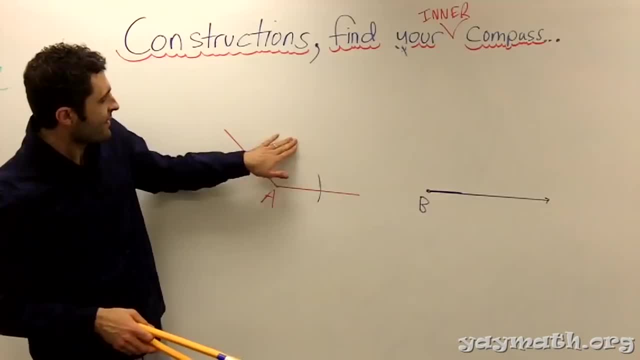 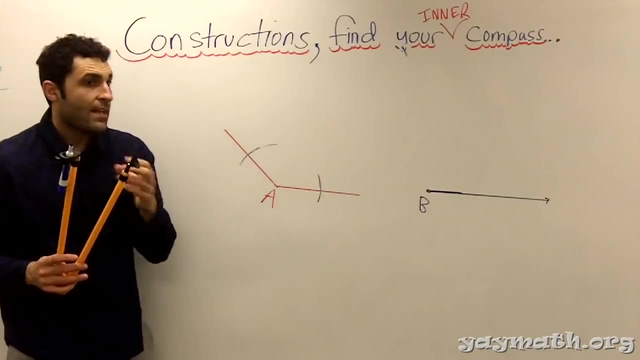 I am loving our time with my wife. All right, Notice. I made two arcs on each of the lines and I kept the length the same, I kept this distance the same, And what we want to do is recreate that over here, Recreate that over here. 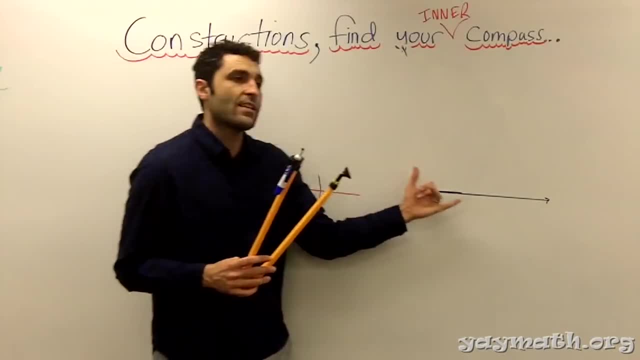 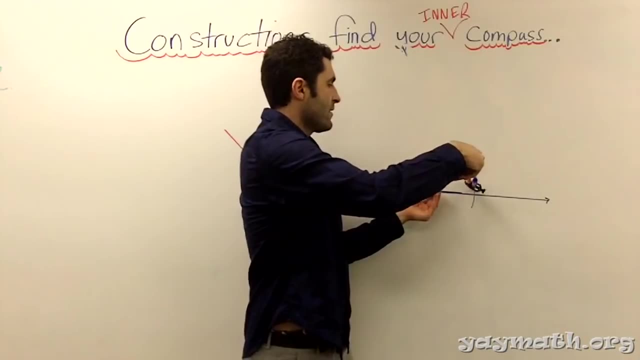 So remember, we put the needle at A. We're going to do the same thing: Put the needle at B And proceed. I have a question, Please ask. So I tried doing that and I made like a half circle kind of. Yeah. 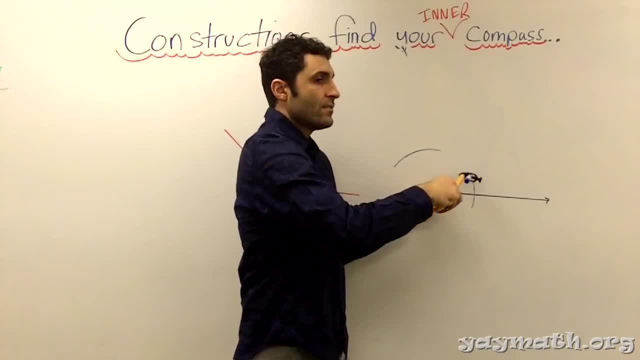 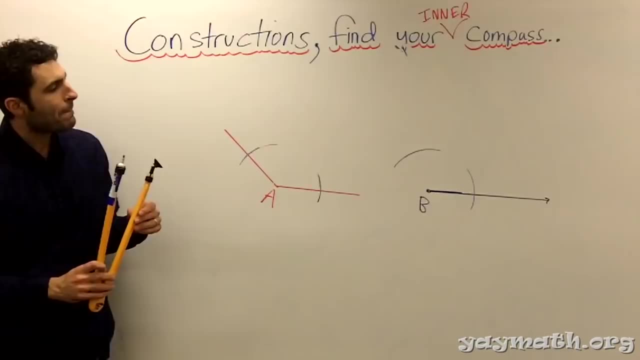 And they're not in the same place. The compass moved, Or the needle moved, Or it changed. It changed. Can I make a circle Like a half circle? You can Wait And so wait. Are you saying that bottom line is B? 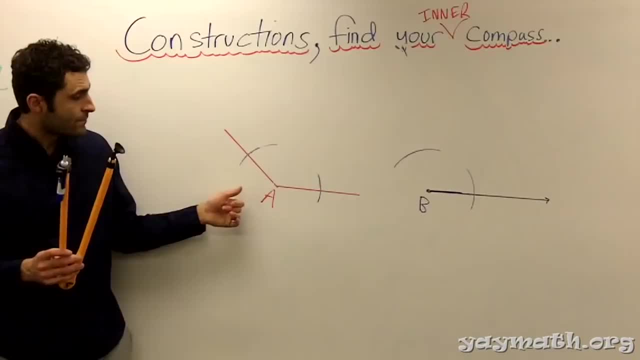 So, like the equivalent to A is B right, A is the vertex and B is the vertex in the future. Is A the vertex of this angle? Yeah, Is B the vertex of an angle that's soon to appear on the board? No, 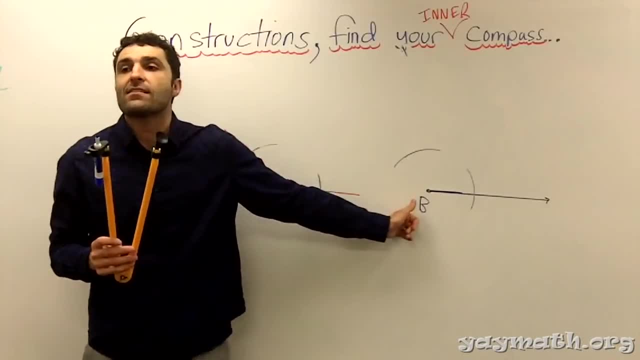 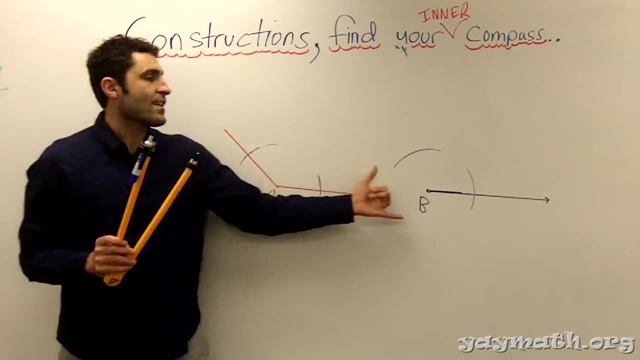 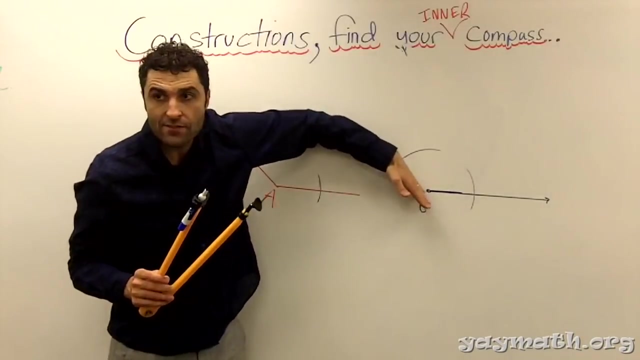 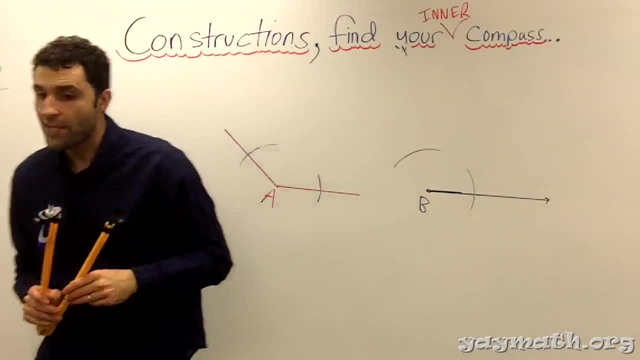 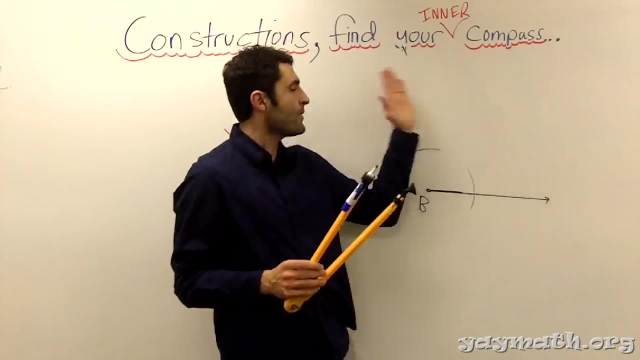 So, Okay, All right, Yeah, Alright, I had to just like decide to draw that with you, Right? Well, what the instructions say? What recreate angle A? Yeah, Construct a congruent angle A. So we need to start with a line. 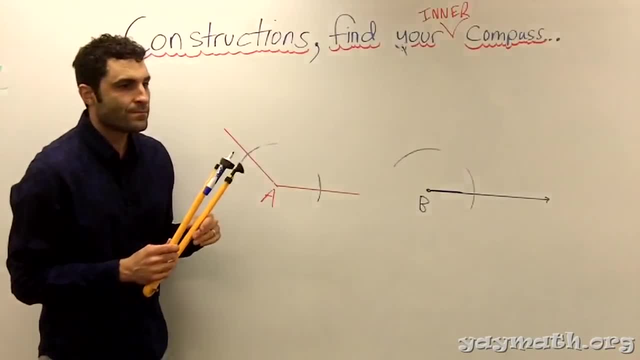 We need to start with some line, And then it's like, wherever you draw the new line, that's, that's as much as the angle is. Can't you just go like this and then, like, put it over near, and then That's what we're gonna do? 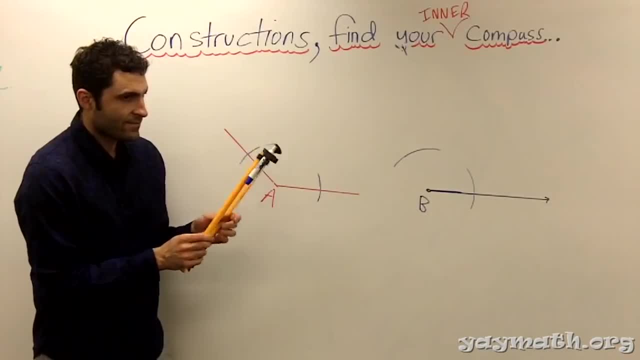 So then we just have to draw a line going through that long line from here: Yeah, That's what we're going to do. So now we just have to draw a line going through that. So now, what do you suggest we do? 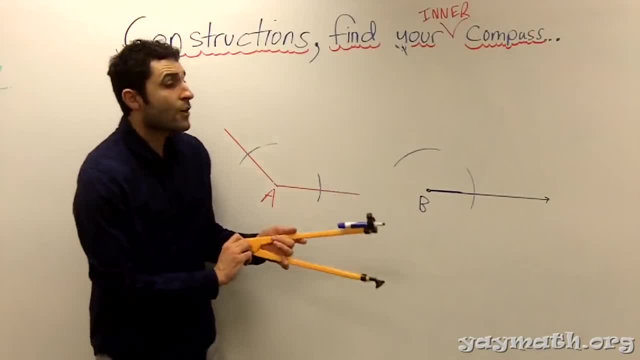 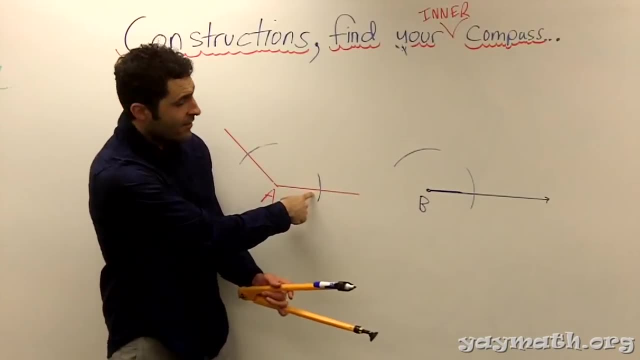 Where should we put the needle now? On one of the new ones? On one of the new ones, correct? Let's start with this one, Because you agree that if we put the needle on this one, then we can put the needle on there too. 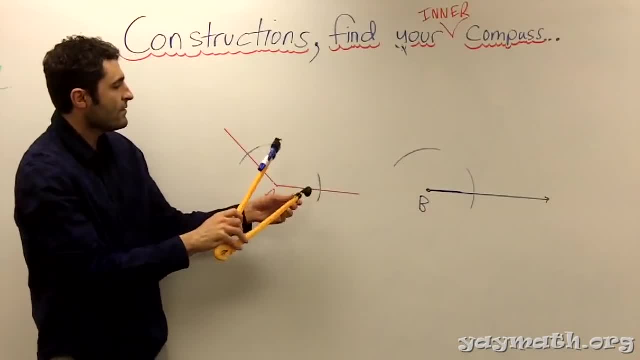 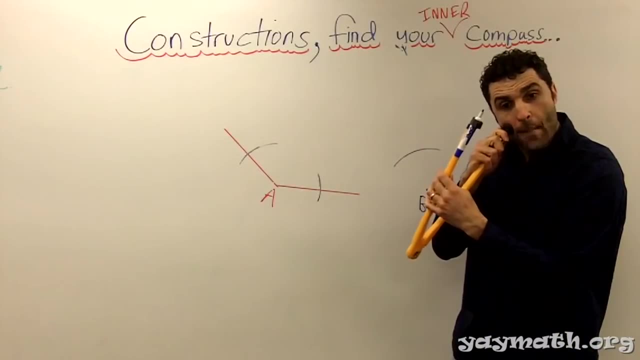 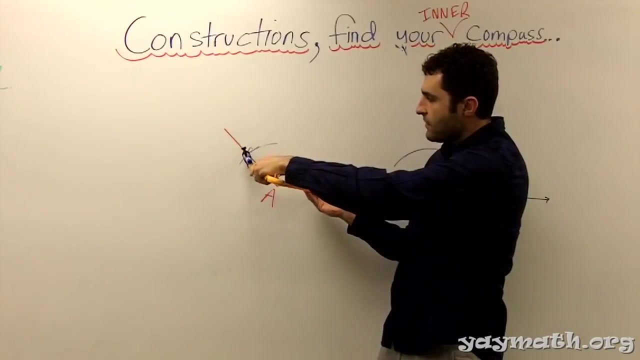 So observe, Needle on this one Stand over here More like a suction cup. I do impressions, So next I'm marking how far the angle is away. See what I'm doing. I don't like this protractor, Okay. 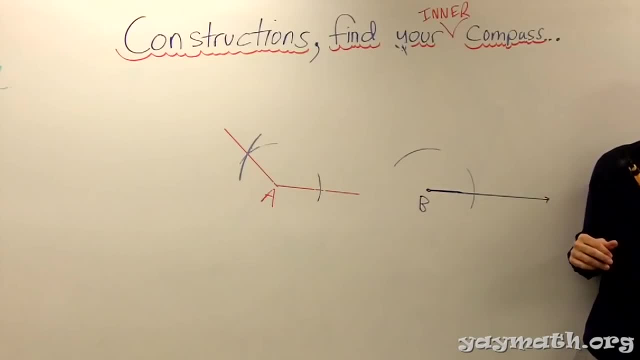 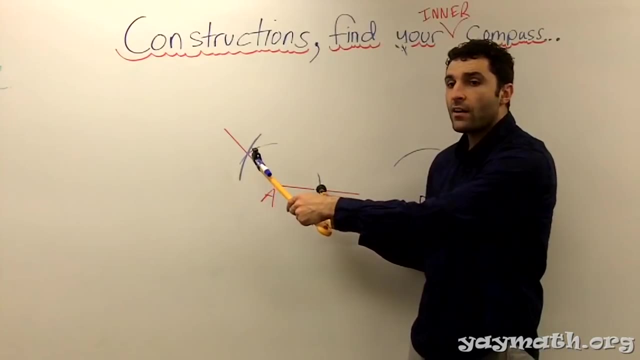 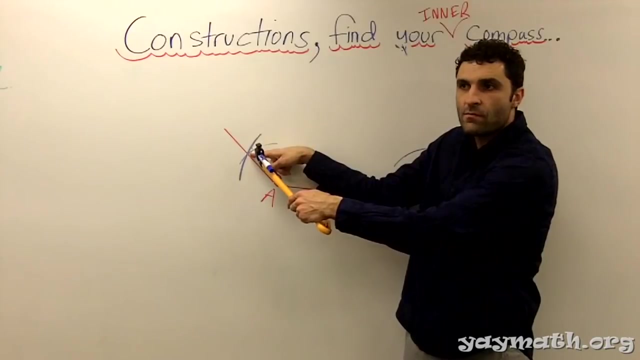 Do you agree that we can only put the needle at points that exist? Is this a new point? Put the needle there And draw an arc And make it longer. The same size, Just make it longer, until you get to this new point of intersection. 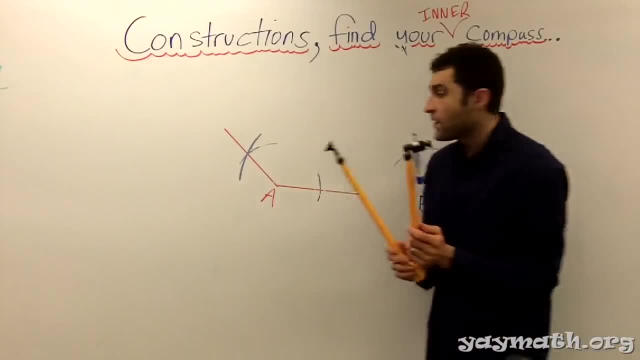 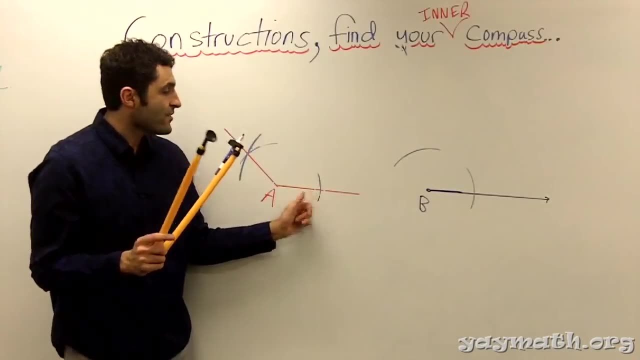 Okay, I figured it out, Do you agree? we created- thank you for asking- two new points with the two arcs that we created. Yeah, Now we can use this point. You see that this point is just like this one over here. 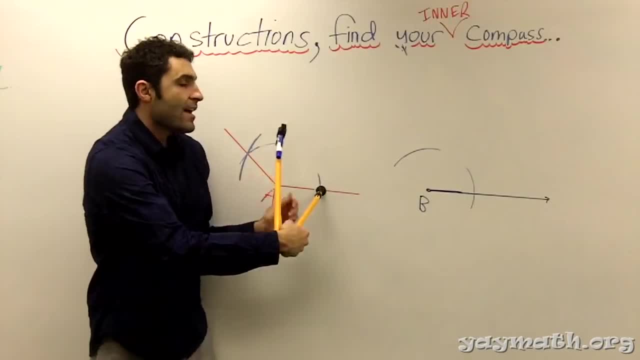 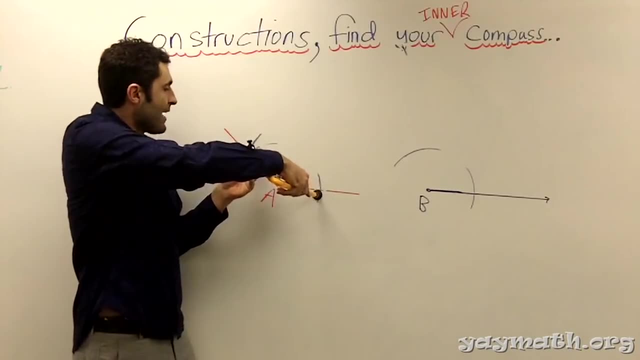 Let's use it. We'll put the needle here And then we say, well, how far, how wide is this angle? We go with the pencil up to that additional point And we draw an arc here. So I have to kind of like: 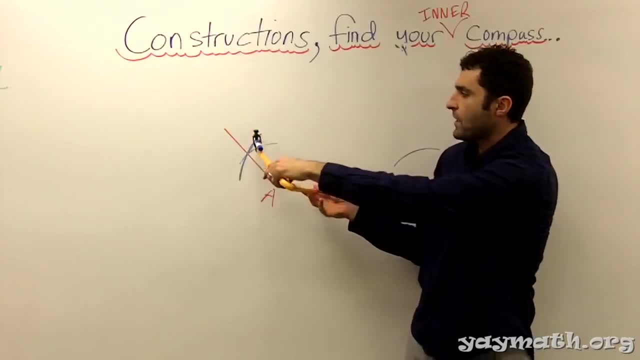 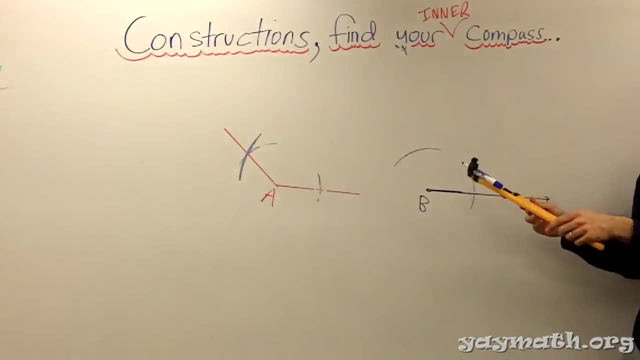 adjust my needle. Yeah, you do Still put it there, but then put it as far as that new, as far as the other point, And then do the same thing, Replicate it, Brother of authentic. Okay, I want my shirt. 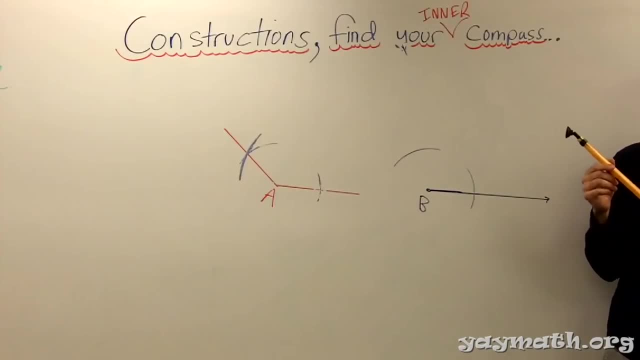 So we're going to do the same thing. We're not like you should call him genuine or something. He's like a synonym. What's up? genuine Sister's like real. No, no, no, no, no. Someone calls him artificial. 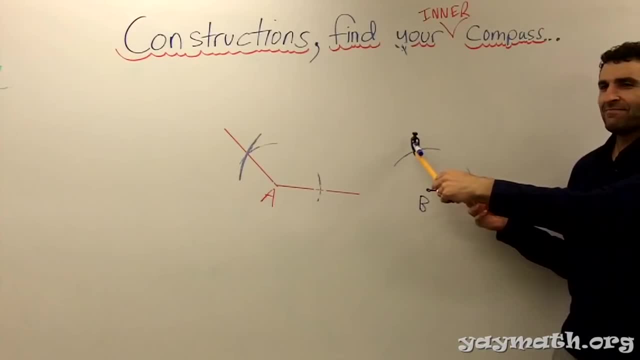 Artificial. It's Antonym Day. Don't listen to me, You're better off. So now I make another arc here. See that I created a point of intersection, Just like we did over here. to here I don't get these arcs. 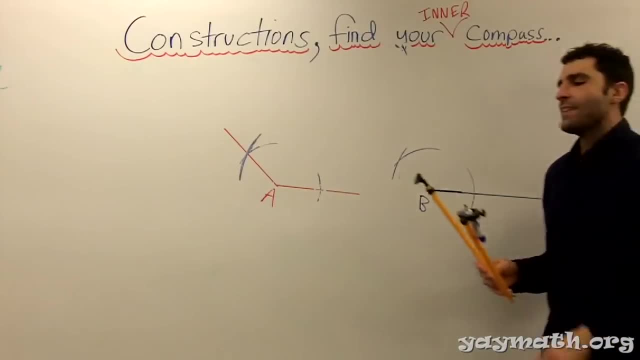 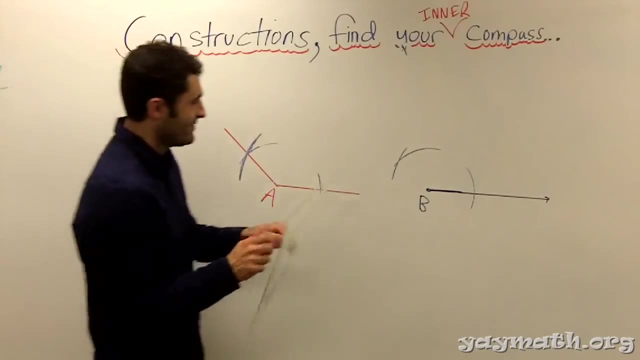 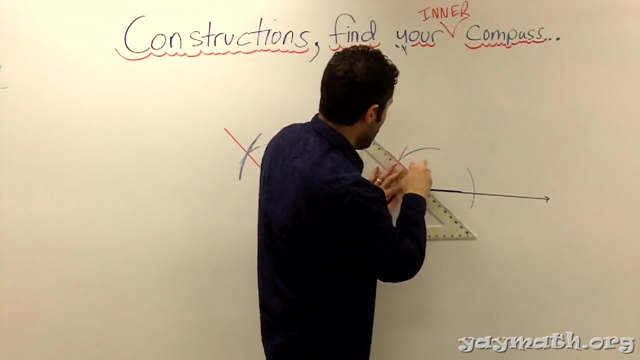 But basically the arc is here, Then you can draw a line and connect. Bravo, genuine Genuine is one of my R&B classics. Can't you just draw that line and go with that line? No, it's not exactly, Ow. 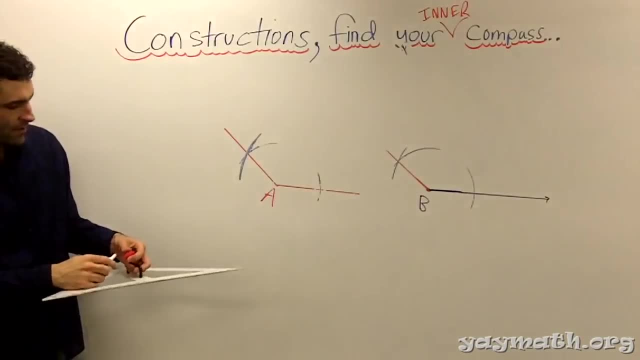 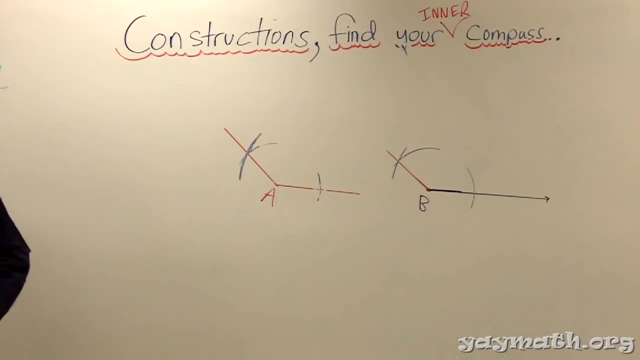 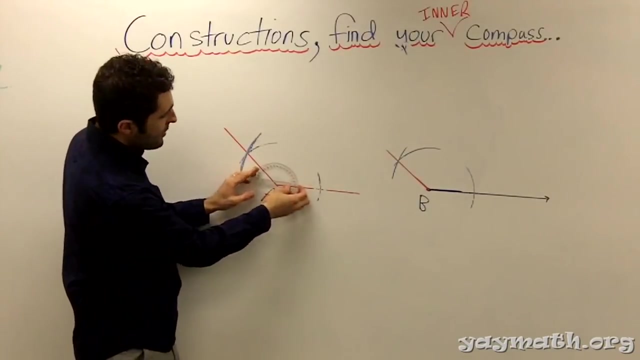 I see the blood. There you go. Mine isn't like that. Stop Now. use the protractor to see. if it's true, Mine's more like a right angle. Then you must have done something wrong, dude, I can help you. 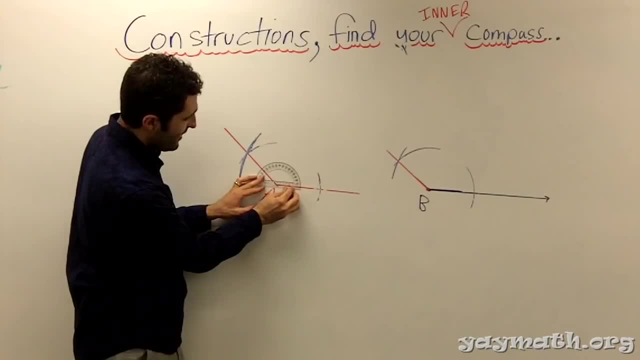 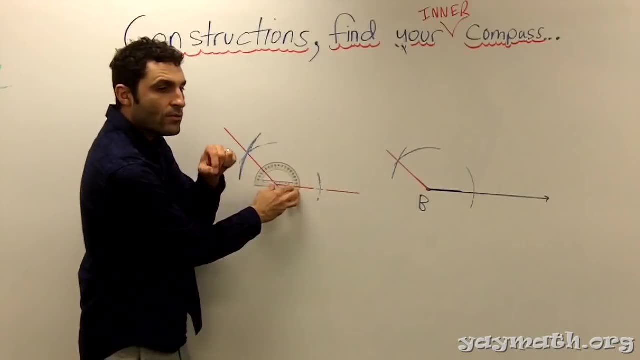 Observe Measuring the original. Can you help me? Don't worry, man, You're gonna get it. Keep going, You're doing it, I see you. Here's how to do it. You put the little hole right at the vertex. 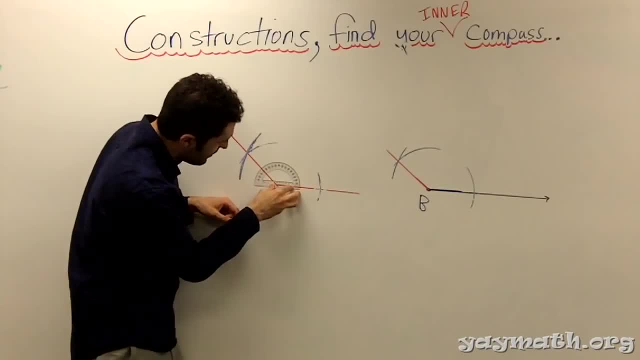 And then the lines that come off, that little hole line with the line you have, Okay, Just right in the middle. You may need to extend the line of your angle to see it, But I think yours is like what, 110 or something. 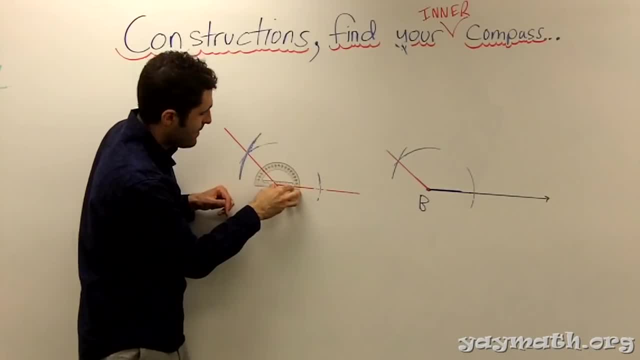 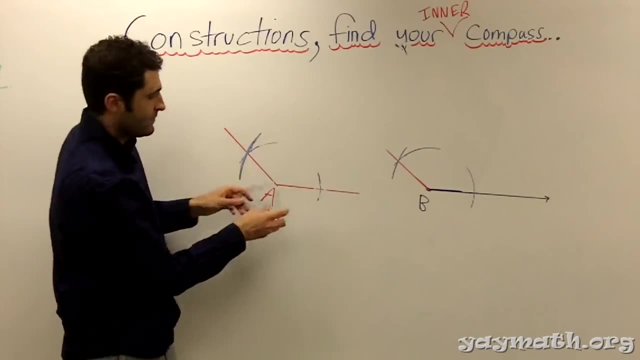 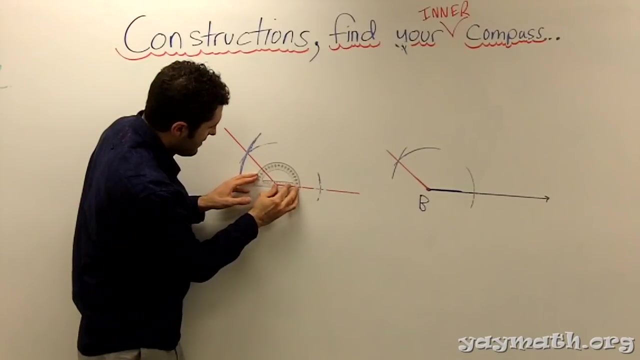 100? 110.. I'm not 120.. You may need to extend the line of your angle Meaning. extend this line- Ah, it worked. And the other one's half, Or the other one's the same, Mine's 120. 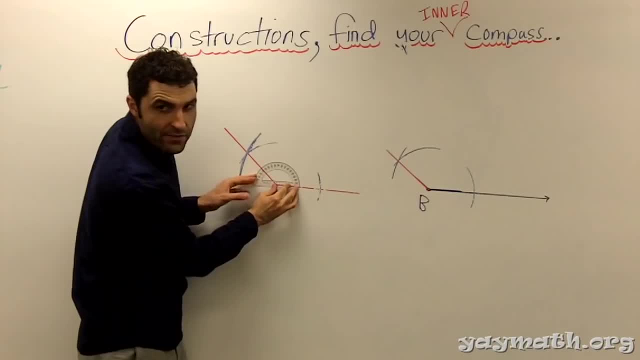 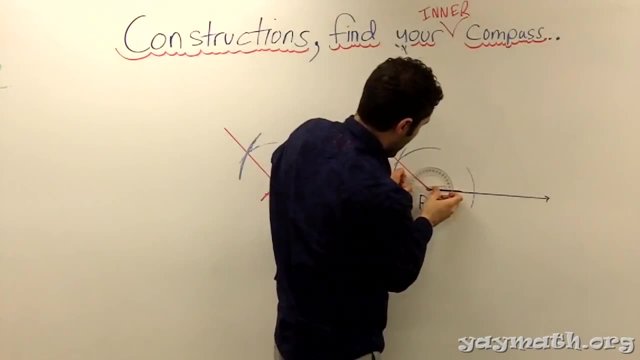 Well, you probably are. It's the same thing. Mine's gonna be 110 as well, Unless some of them. So I got like 140 here. Wait, I don't get it. And mine is 140 again. 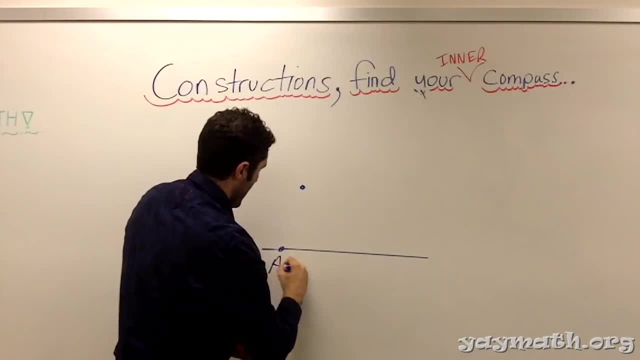 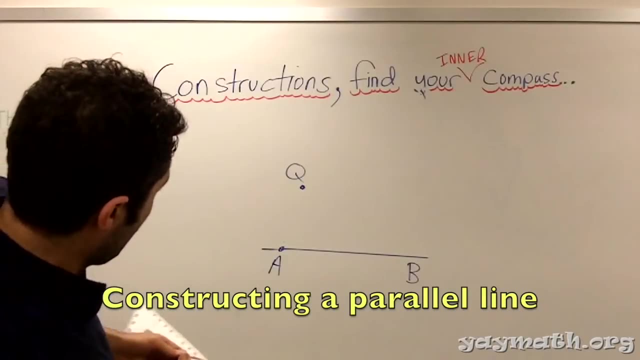 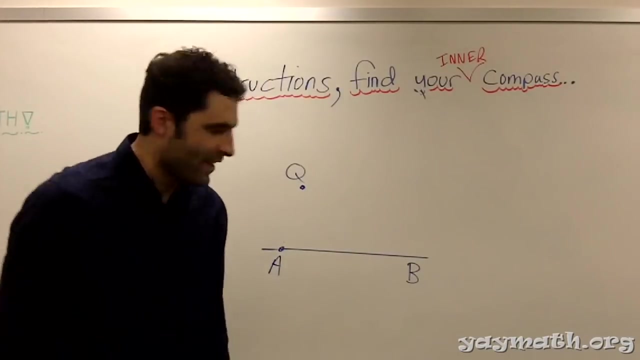 Yeah, 138.. I give up, Maybe, Maybe slanted. Yeah, If you slanted it, they're alright, I'm okay, It's good enough. It's like slanted when they're long. Does it matter where Q is? 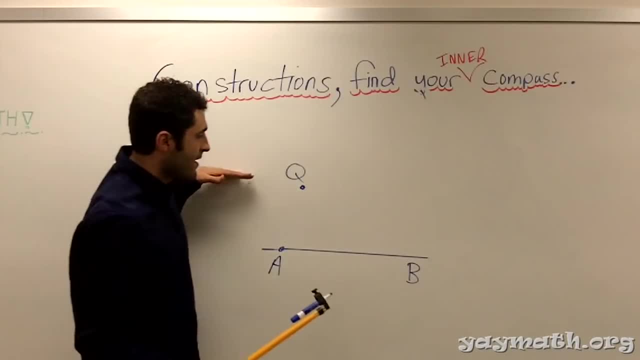 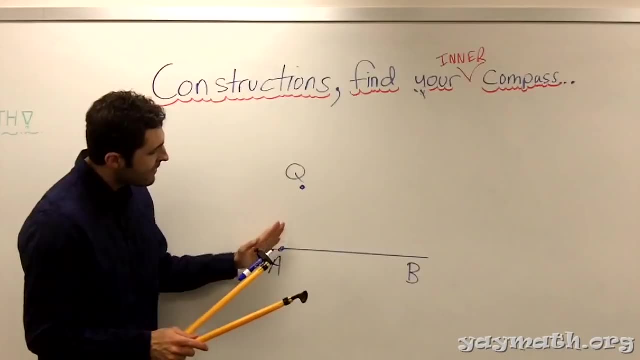 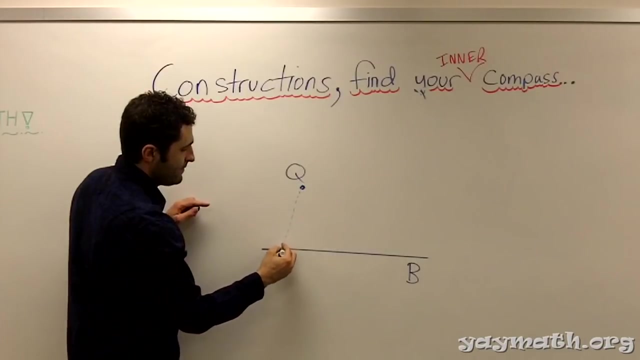 I think it's okay. We're going to make a line parallel to AB, that's going through Q. Now do you agree that, if we have? Ah, I want to give you the hypothetical. The hypothetical is if I were to draw this angle. 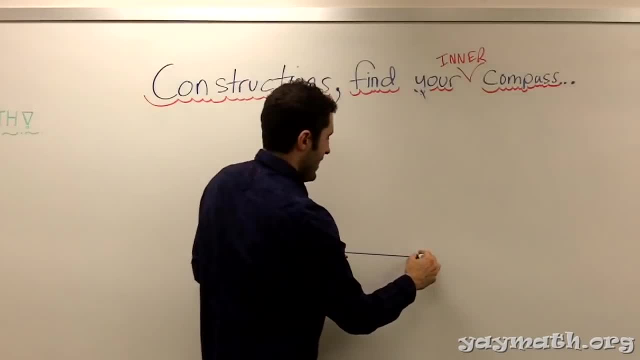 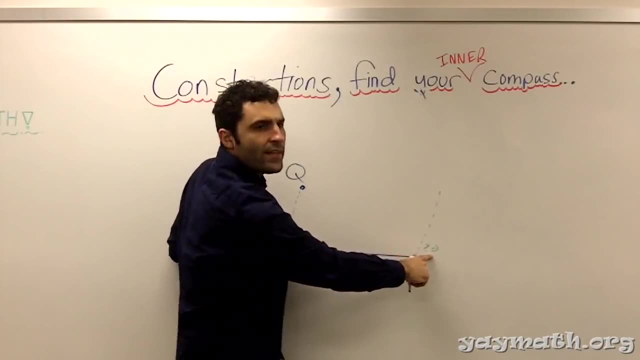 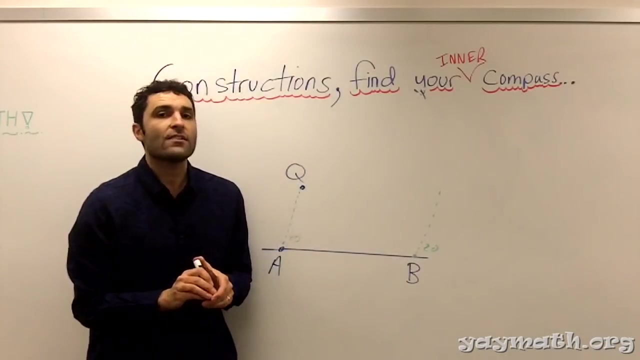 let's say it's like 80 degrees and I were to draw this angle, and if it was 80 degrees, then these two angles are called what? Kuguli? Parallel. You guys are all on the right track, Corresponding. 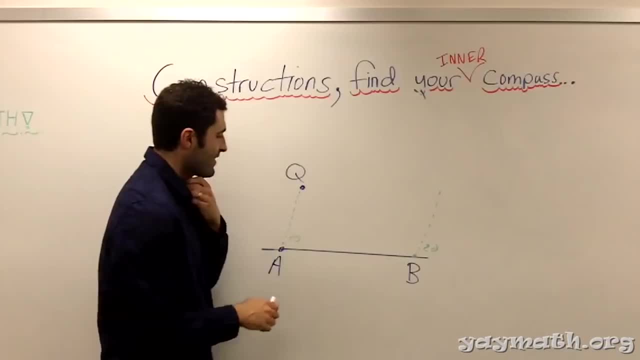 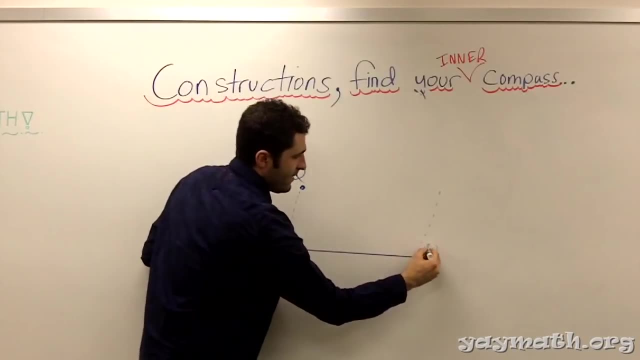 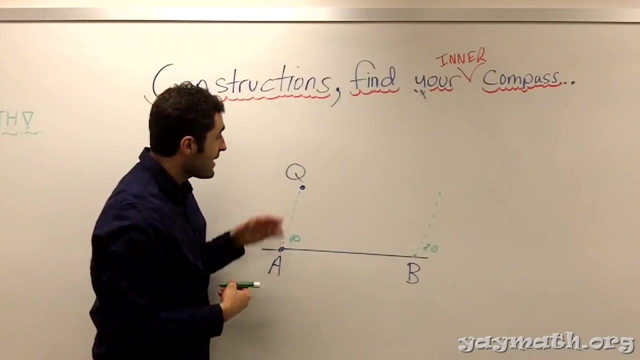 They are corresponding. They are corresponding. They're both in the top, right, Right. This is 80 and this is 80. So if we can make angles corresponding, then this line will be parallel. So let's, Can we just make a triangle. 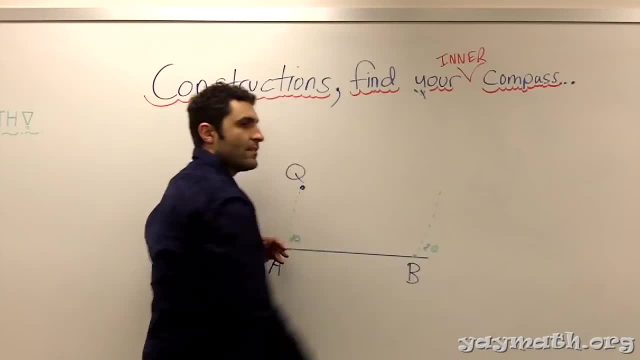 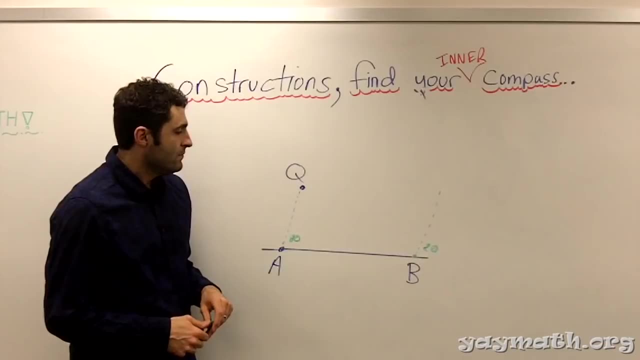 Well, if we made a triangle, how would that help us create a parallel line? We could make another triangle, the same triangle, on top of that triangle. Oh, I thought you were trying to make a line going through Q and splitting AB. 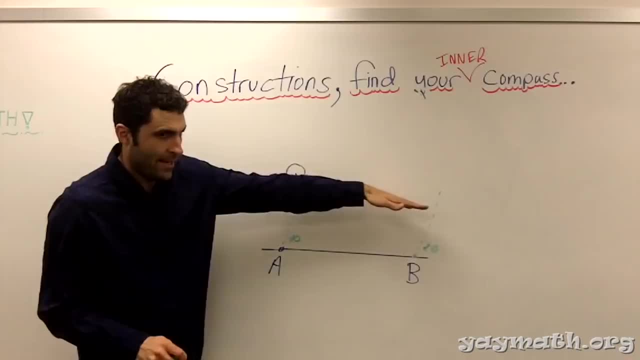 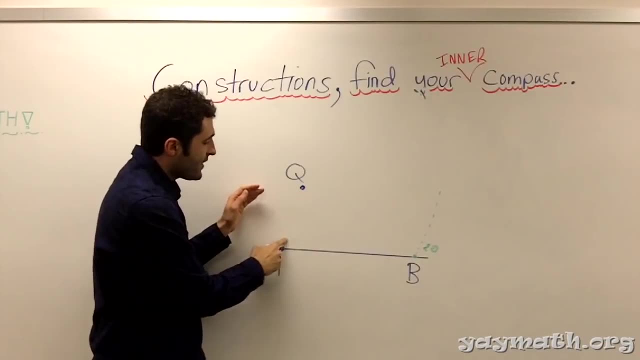 No, that's another one. This is going parallel to Q, Parallel through Q to AB. So let's recreate angle QAB. Let's do that now. How do we recreate angle QAB? You get your protractor and you put it on Q. 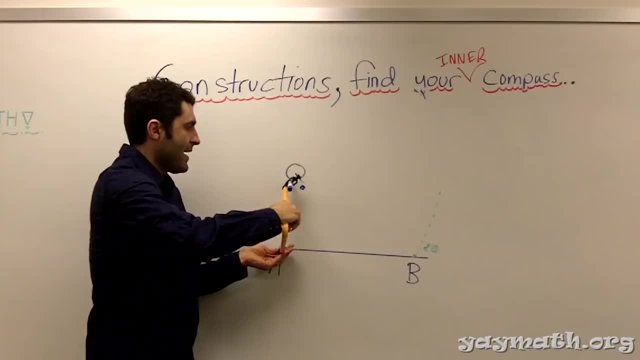 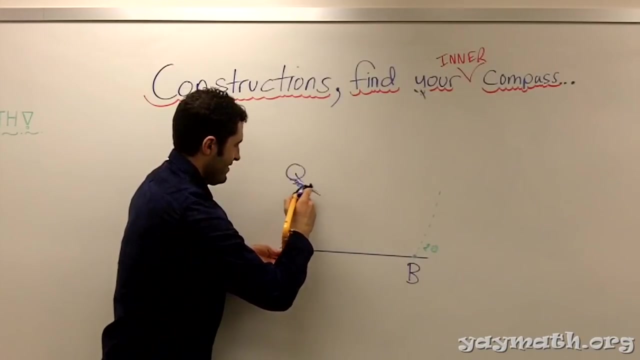 No, you put it on A. Put it on A And we have another large. Here we go. Did you put your arc on Q? Yeah, What's wrong with my homie Cool line? Wait, do you want to draw like an X? 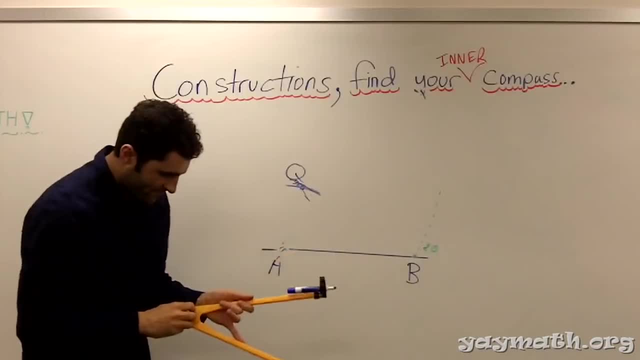 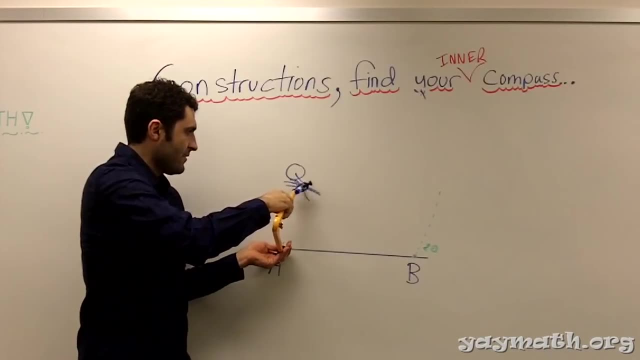 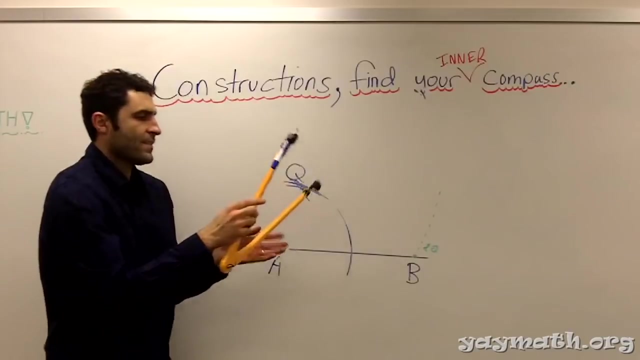 Do an arc If you can do it better than me. I don't think we've ever covered this much. There we go. That's an arc here, and then down Here, and then down There you go. Keep it the same. 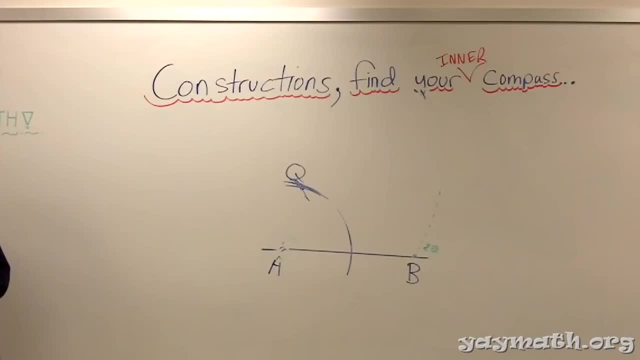 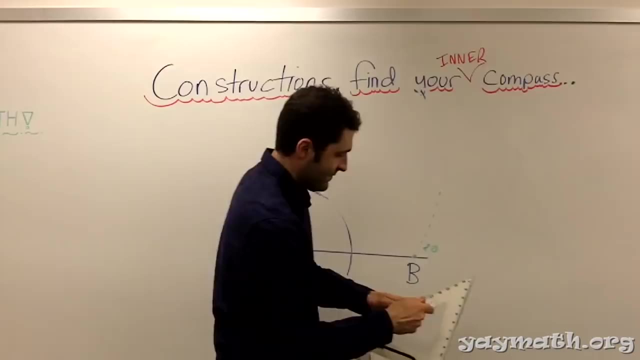 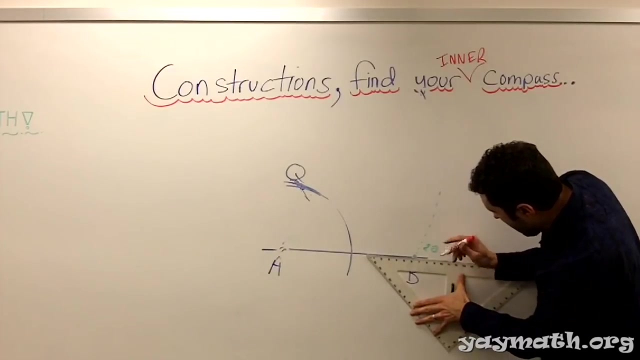 Keep it tight, literally. I will need to. Where's my red? I'll need to extend the line. brothers and sisters, Extend the line. Are we making a circle? You can make a circle. I noticed that I did. Do we need to extend the line? 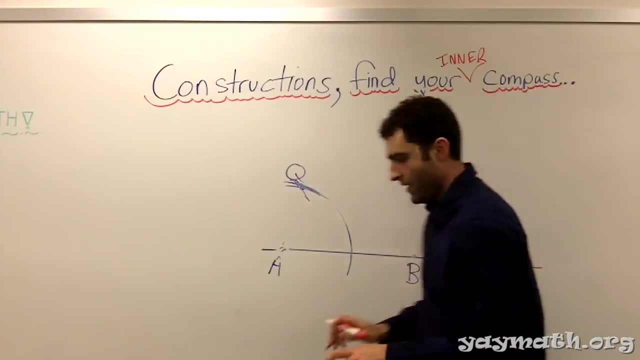 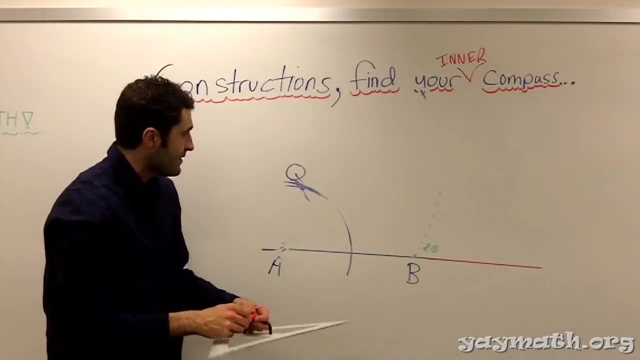 Yeah, I think you do Peace There you go. Wait all the way down, All the way to the end of the page, Because we're going to make another angle. yeah, We're going to make this angle again. Bless you. 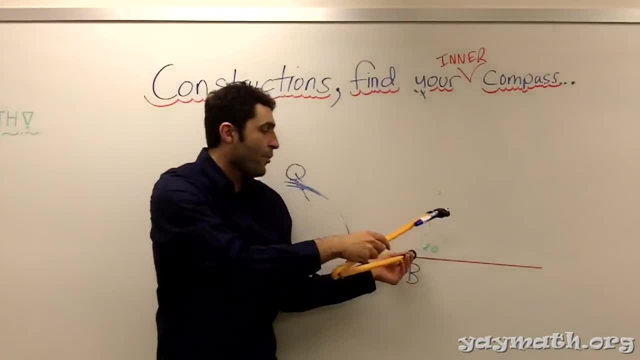 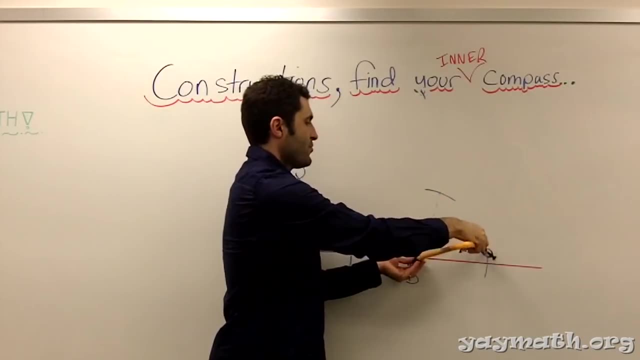 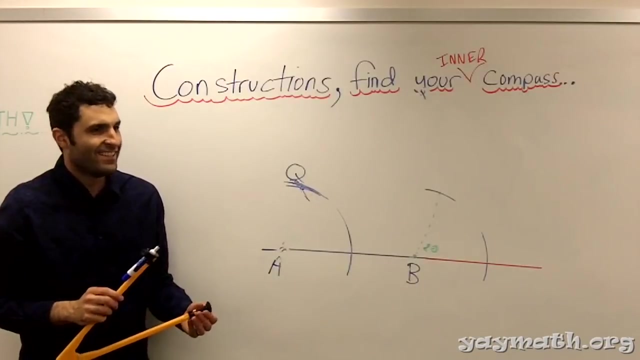 Bless you, darling. And now we're going to do the same thing. Point at B arc and then arc Pointy Noah, two giraffes. We just made an arc reference. Oh, That was a good one. 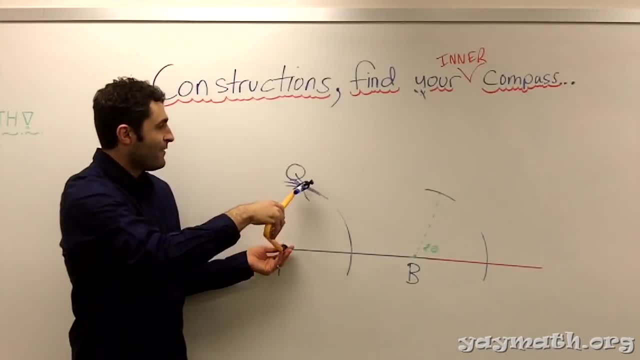 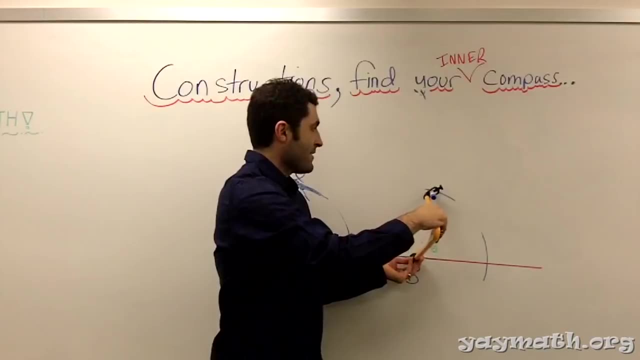 Thank you, You're welcome. Get on there everyone. But in this case we're making two arcs, So you know, now we can bring your cousins, not just two of them. You keep the same length, right Yeah, same length. 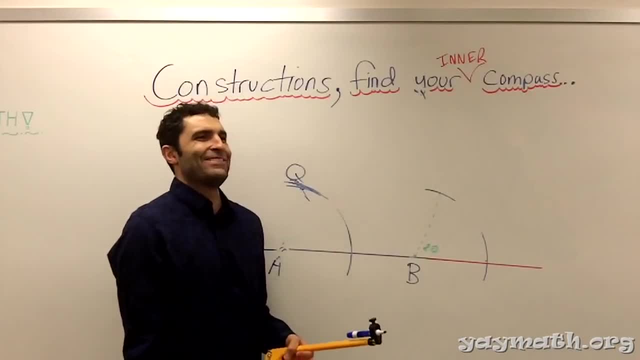 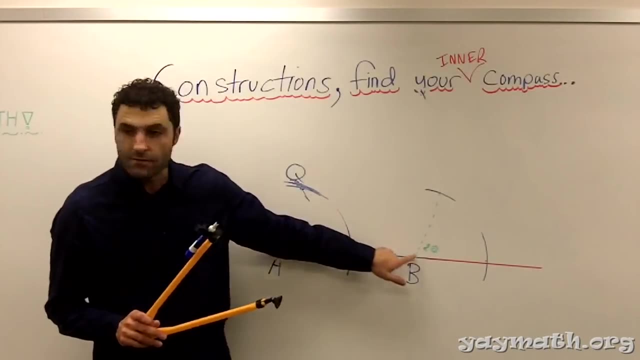 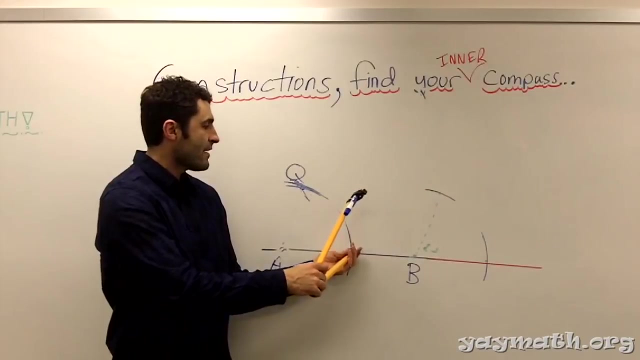 You just made it funny actually. Yeah, remember when you docked your phone? Yeah, Oh, I didn't measure it. I didn't measure it. Next New point created Here: How far is it to Q? Let us find out. There it is. 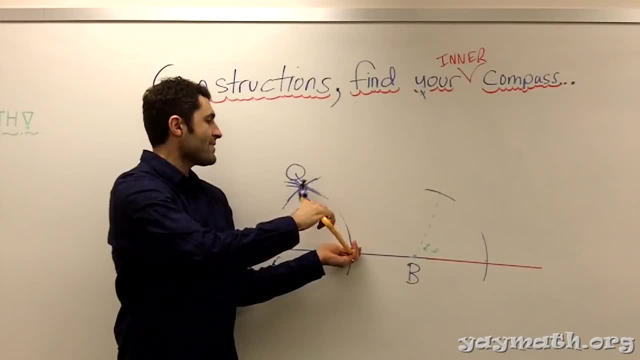 Not far enough. Not memorize, Learn. We're not having a test on this. Not memorize, Learn. So notice: we created a new point and now we go to Q with that point. Wait, do I extend this? 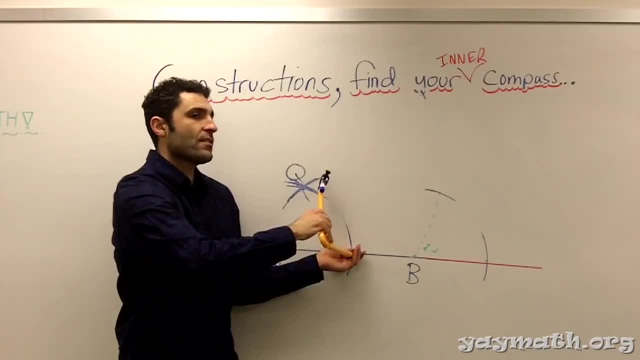 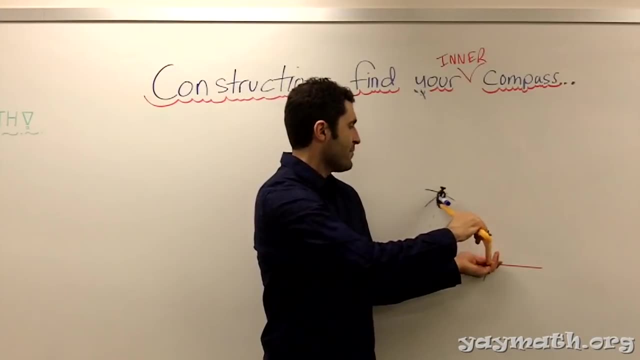 Yes, extend of course, measure how far it is. Then again over yonder, hit, over yonder. over yonder. Look at that, See that. So I created another arc. Look, I did it over here at the new point. 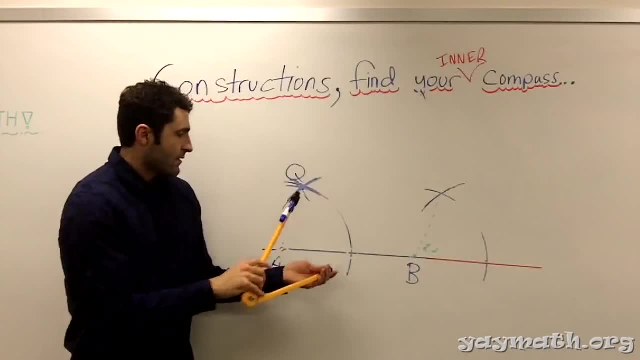 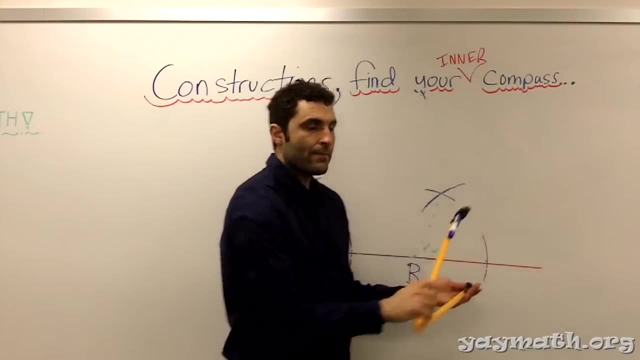 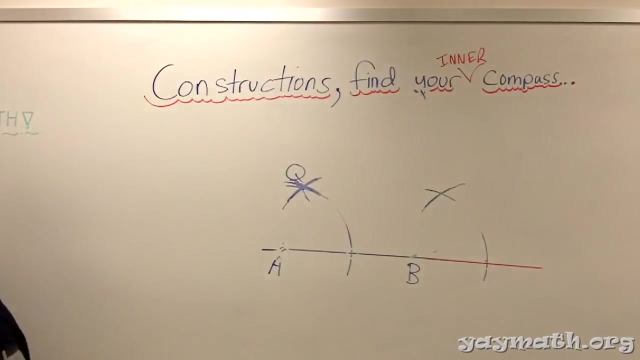 You did the point on A on that line, Yeah, so just like here at the Q. and then this new point to this arc out here: Okay, Is that tonight? No, it's Thursday. Now I didn't get that. 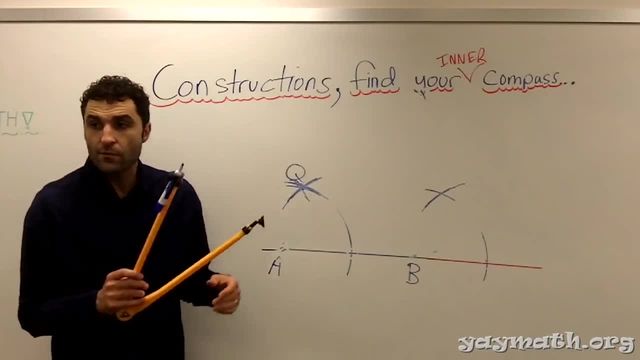 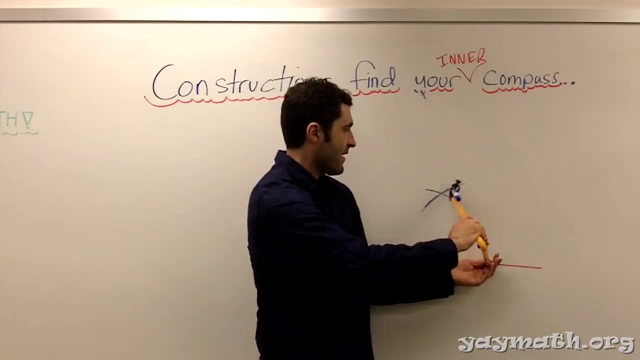 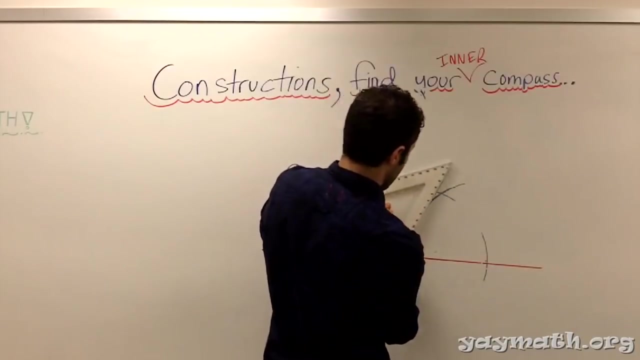 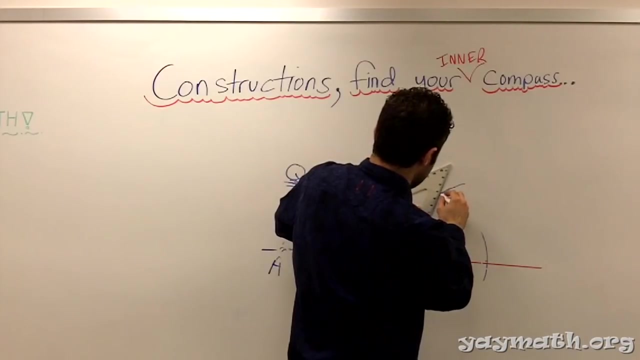 Okay, Do you know the process? What's your process? Did you go from here to here, Make an arc, and then from this to there? Oh, do you connect? Connect You like. So now we don't really need to. 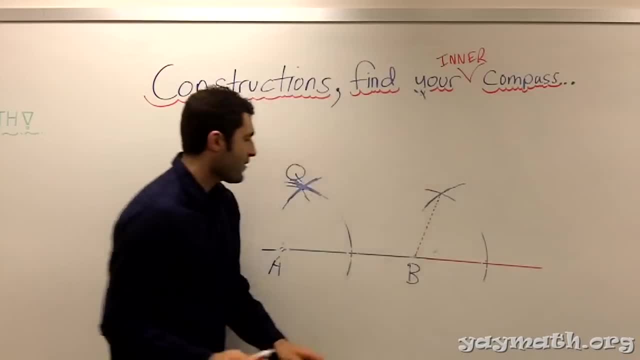 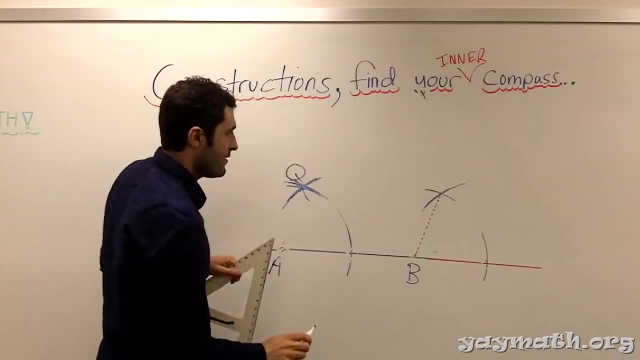 it's not the angle that we're looking for. Now that we know that the angle is the same, oh, I erased this. Wait, you go to A. You go to point A. Don't you just go straight down From where to where? 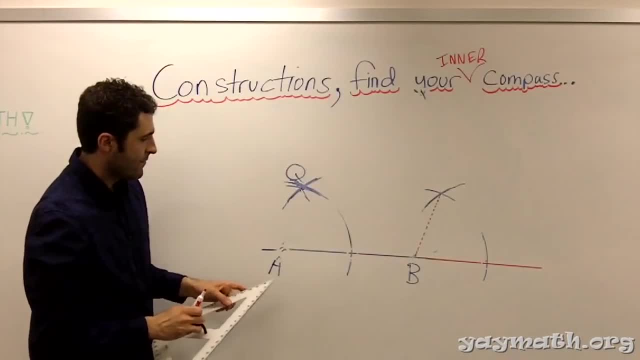 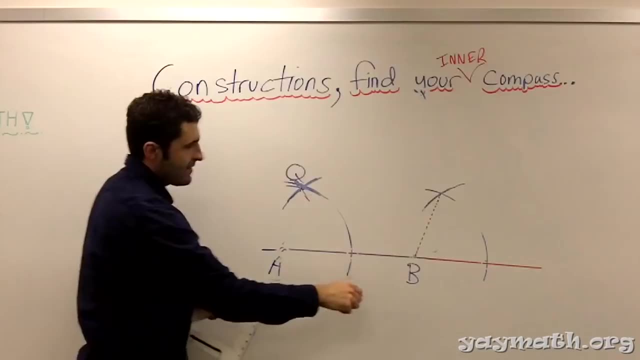 This is what we're gonna do. Yeah, I know, but don't you go straight down from Q to A? Not necessarily What we want. now that we know, do you agree that QAB is now the same as this to B over there?